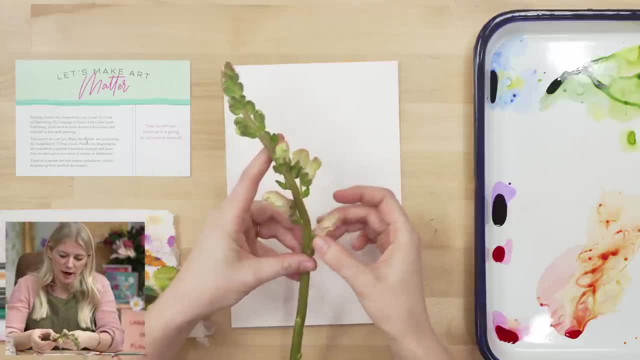 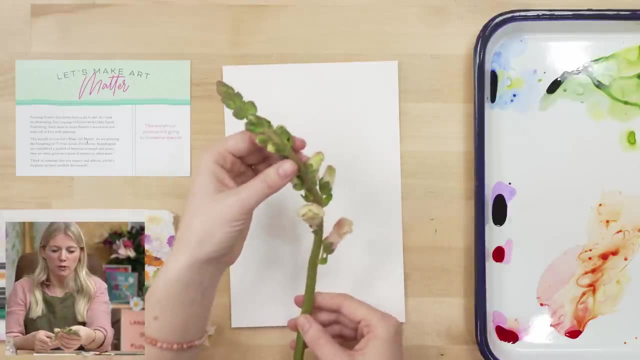 it's on a thick stalk and the flowers come out individually along its side. The thing that we have to pay attention to is that this stalk is three-dimensional, which means that there are flowers on the sides, on the back and in the front, So we're not looking at painting a thick 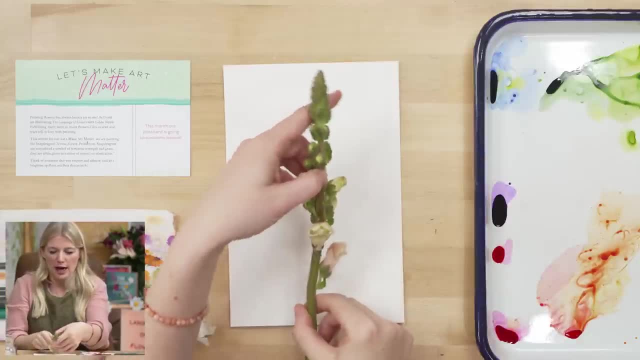 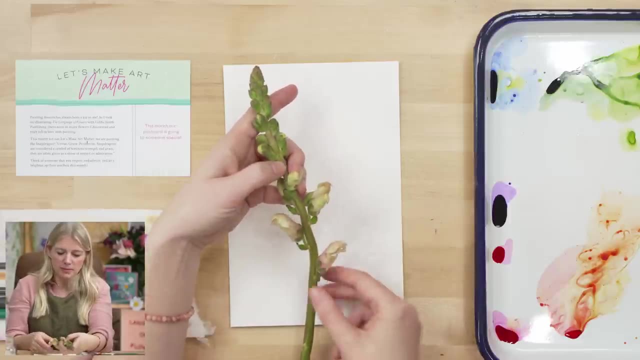 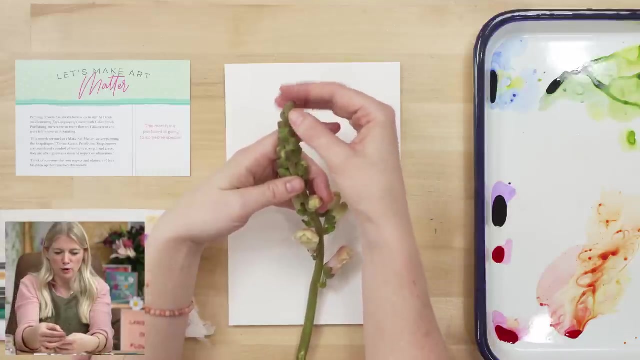 stalk and then flowers on either side, because that is not how it actually is right. They go all the way around. The other thing to pay attention to is that the blooms on the bottom gradually get smaller as they go to the top, where it kind of ends up being these small green. 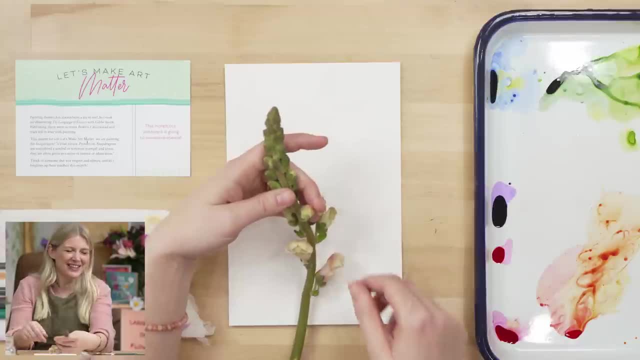 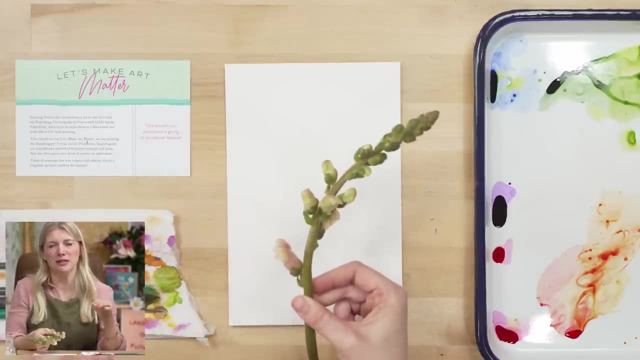 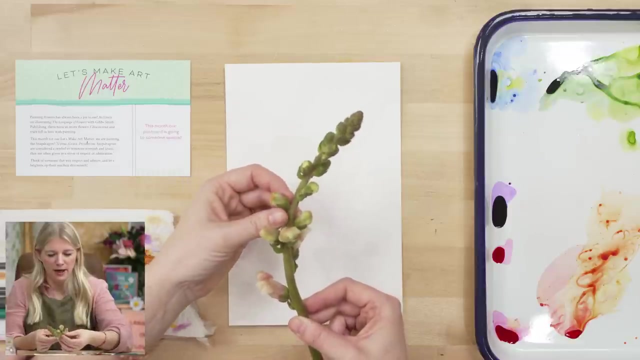 kind of like pods, Buds, Buds. thank you, These little buds along the top. okay, Now the floral shape itself- and there are different stages of blooming, so sometimes they're just rounded like this- is starting to come out from the bud, but it's still just round and tight. These ones are still. 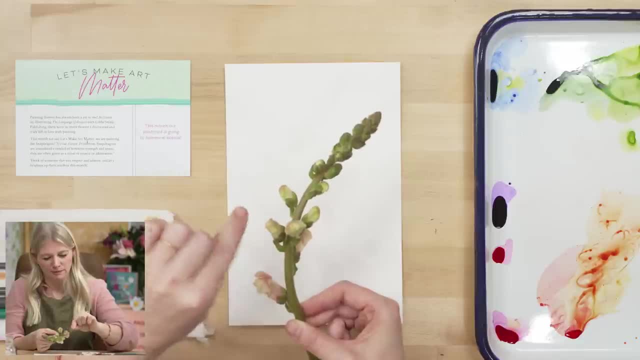 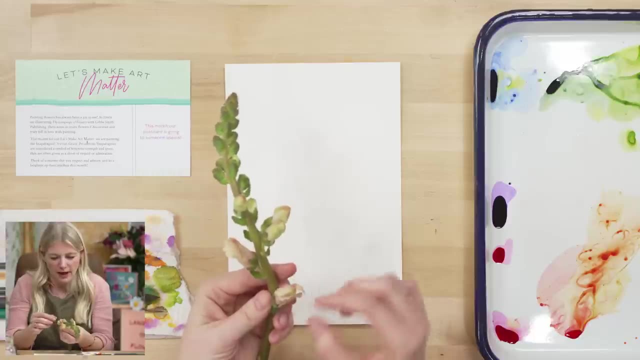 pretty round, but they're kind of elongated And they have like a little fold right here. and then these ones. you can see that they're starting to open up and I'm going to like just press these a little bit more so you can see what they look. 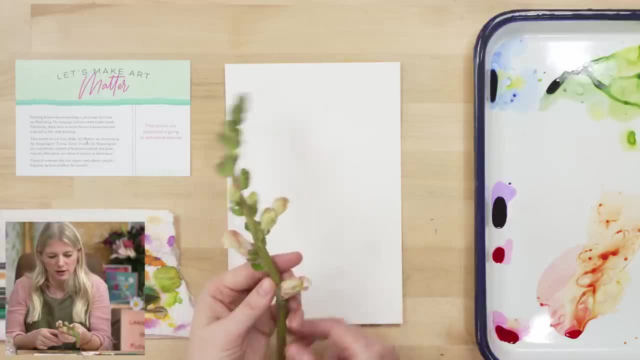 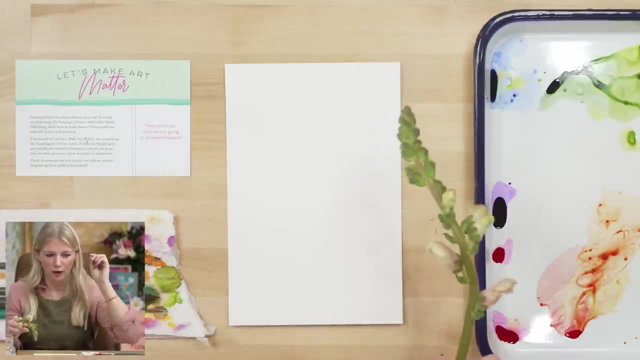 like more opened up. okay, They get really papery, like if that was an older one. the lower flowers get big and mellow and papery. Yes, so we are going to. when we recreate our snapdragon, we're going to think about all of those things as we're painting this. Now, I'm not going to paint this exact one. 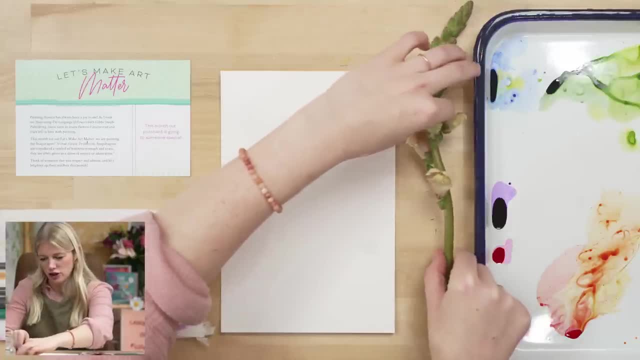 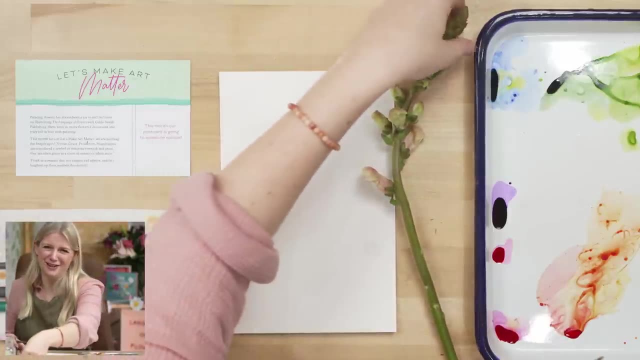 because I don't want mine to have a lot more flowers on it and be a different color. but this is just a good visual for you guys to have as we're painting these. And who doesn't like fresh flowers? I mean, come on, they're just lovely to have around. So I'm going to start with my round. 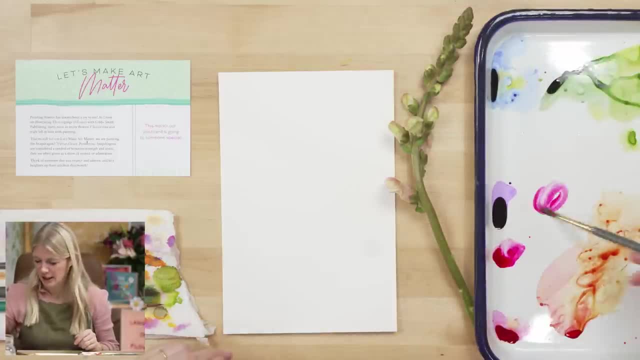 six, but you can use whatever brush you feel most comfortable using. I'm going to grab some magenta and I like a really peachy blush color personally, but these come in all different colors, so just use whatever you feel comfortable. So I'm going to take my yellow and mix that in with my magenta to get this really gorgeous kind of. 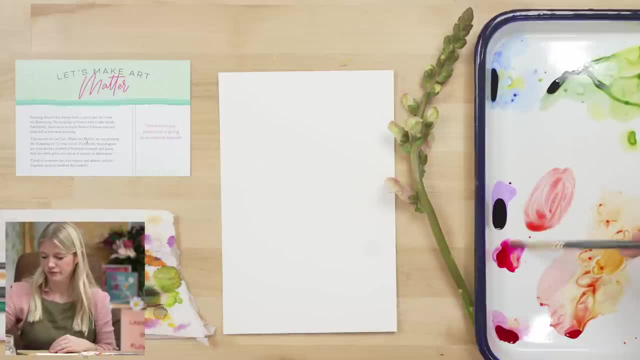 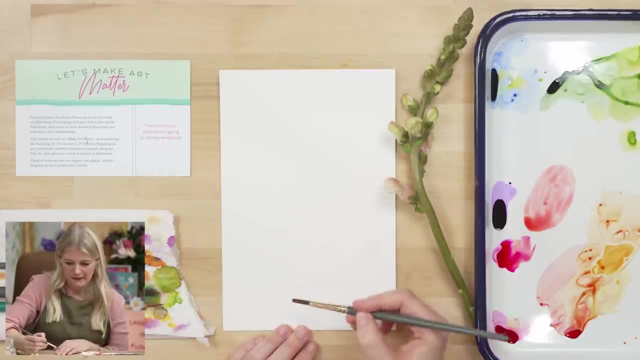 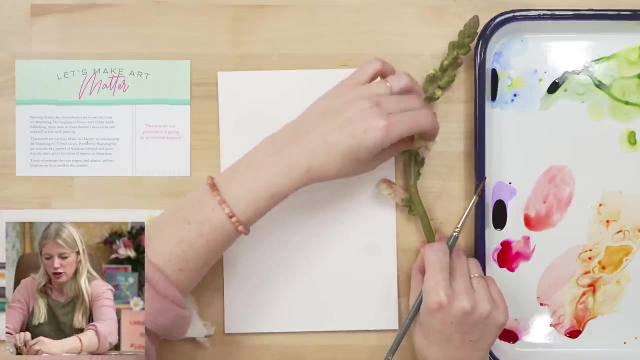 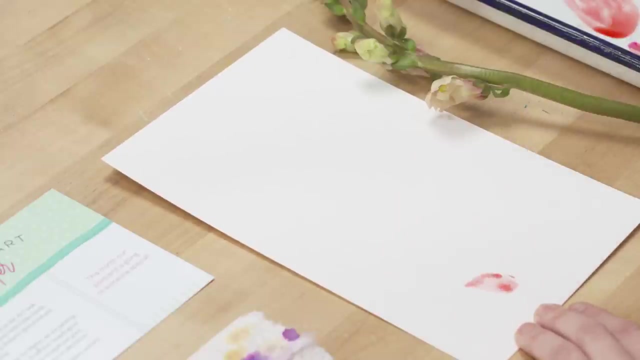 coral-y color, maybe more like a salmon, and I'm going to basically think about. they can be going up, they could be going down, but they're all kind of this like roundish oval shape- okay, Like round oval, round oval- and notice that they're getting a little bit smaller. 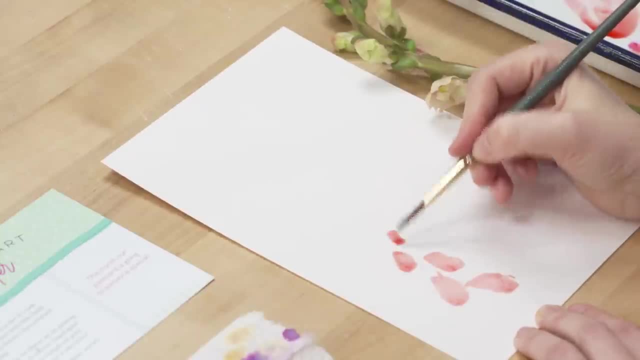 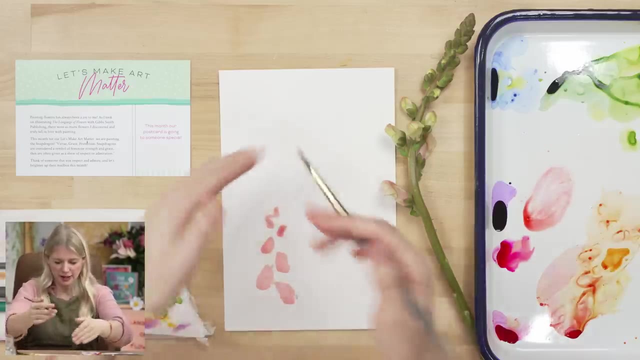 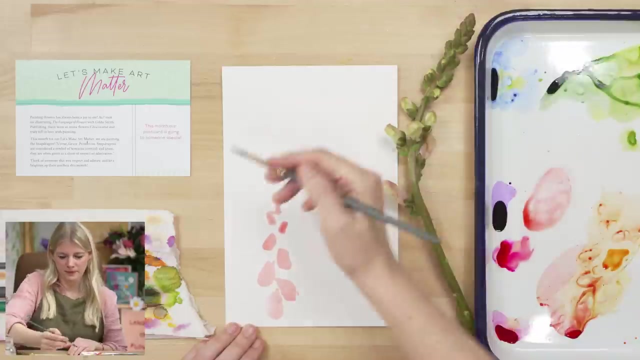 as I work my way up And then maybe now they start to kind of poke out And notice I'm saying this to myself, I did them on each side and that is not true, so I need to do one in the front here. Okay, and then let's let these kind of 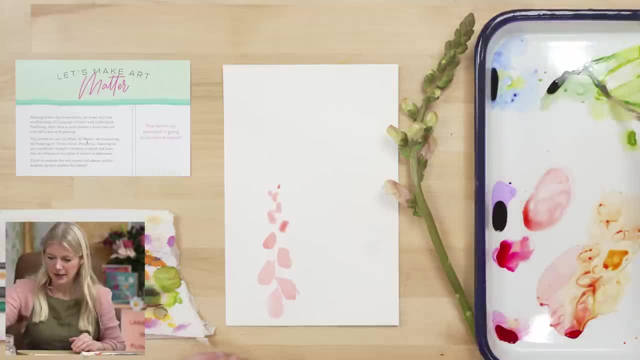 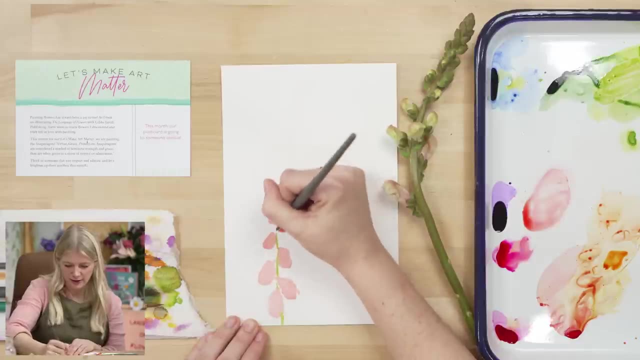 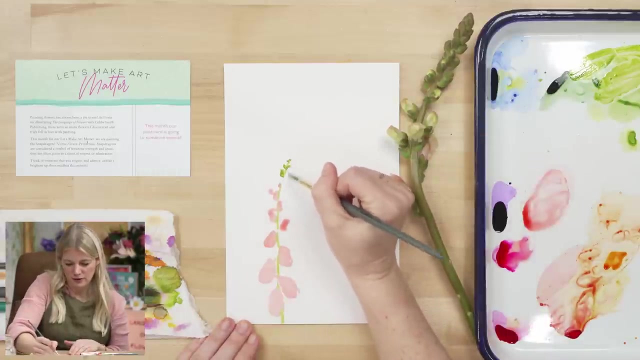 blooms go here, and now I'm going to take my green and then I'm going to imagine the stalk going in between these and then it curves, see how it kind of moves, And then now I can put in those little buds and then touch green to the base. 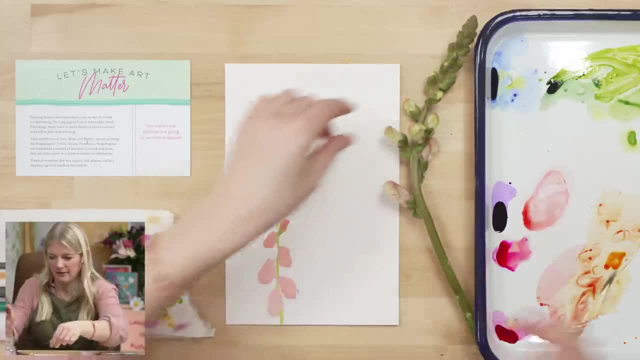 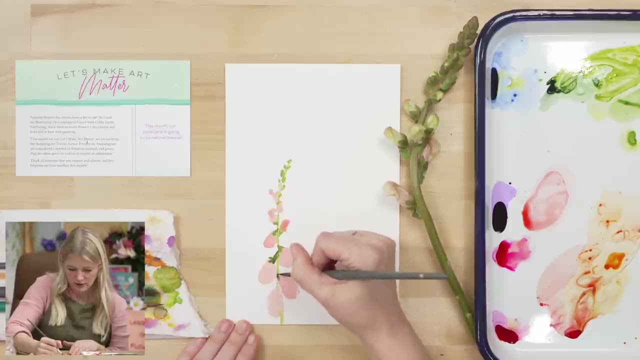 of some of these because you can see that they kind of separate and have like little leaves around the base of it. So they're called snapdragons because their face kind of looks like a little dragon Uh-huh, And you can squeeze them and they'll open and close, which is the most fun. 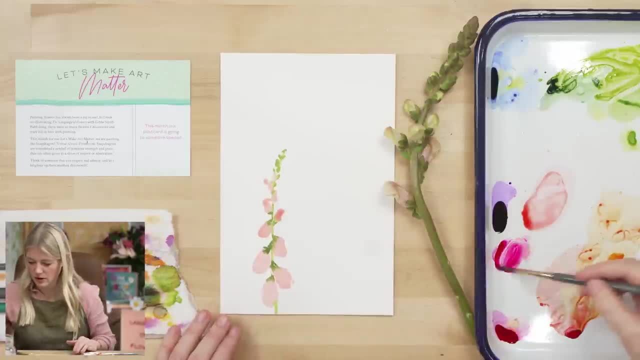 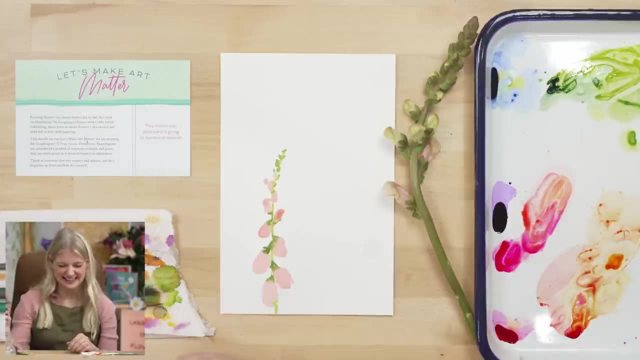 Yes, Their scientific genius is anterinum, which means snout. Oh really, Little snout flowers. That's cute. And then what I like to do, that's such a cute little snout, and then you can leave them soft like this, or sometimes just for fun. 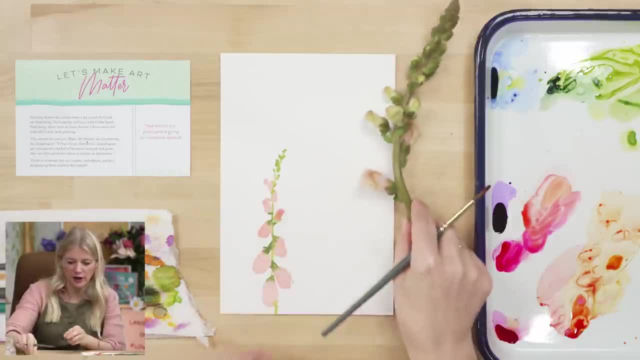 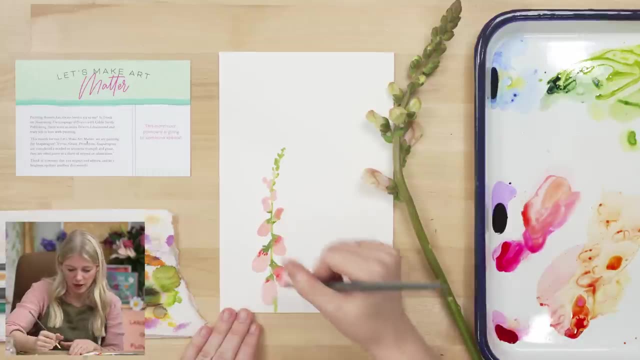 Like because if you look they have different colors going on, so right at that base you can add a little bit more color. Maybe you want to do yellow instead. You can do yellow kind of. maybe that center is opening up a little bit and you can see. 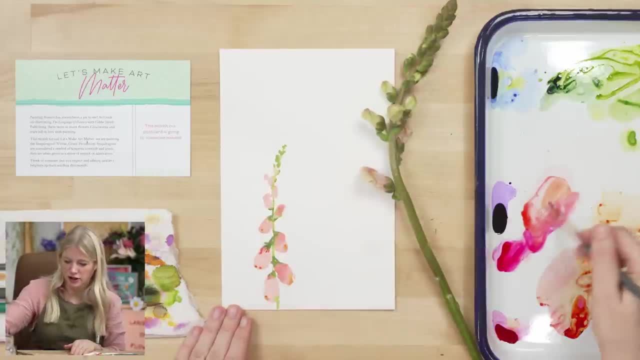 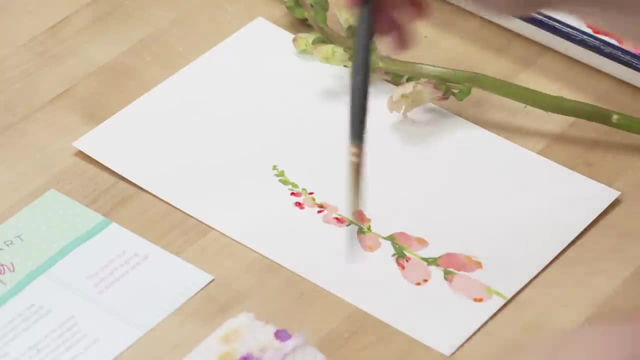 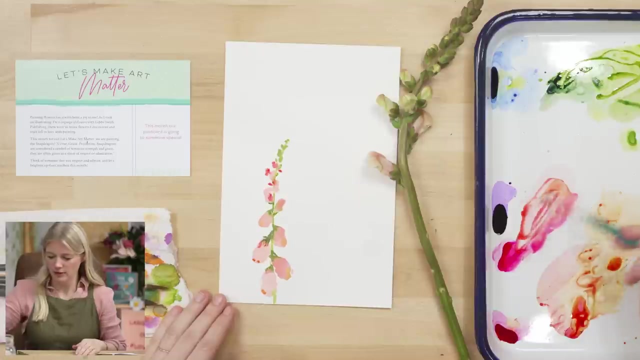 a little bit of yellow, Just kind of like drop drop in some different colors. Let it be a little bit loose. And then the very last thing I like to do is I want to give a little bit more hint of its shape and the little folds that you would see. 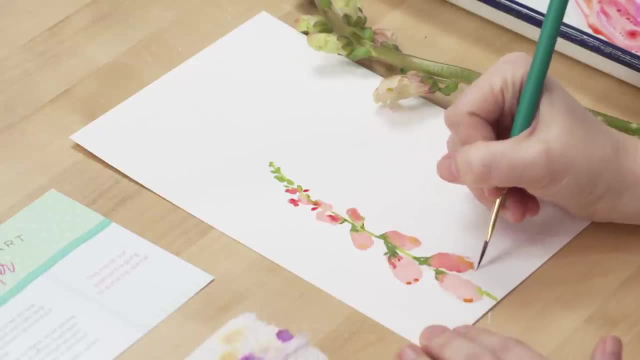 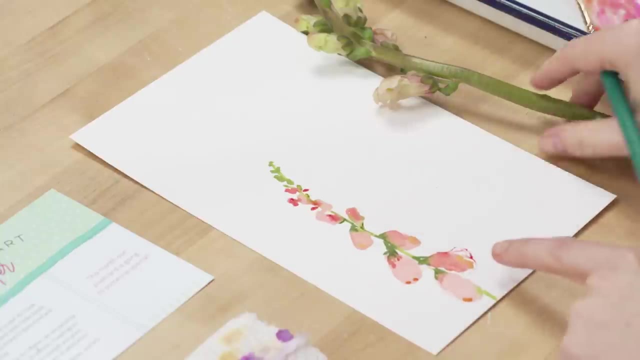 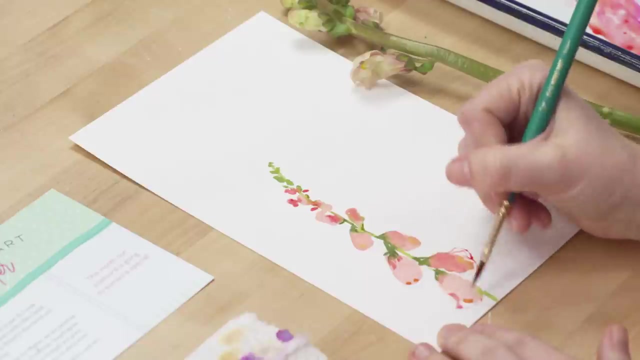 So I'm going to take my dagger and then I'm going to just kind of like draw around it. So sometimes it kind of like that little balloon. you see this kind of uneven edge, Yes, So it kind of like widens up at the top. 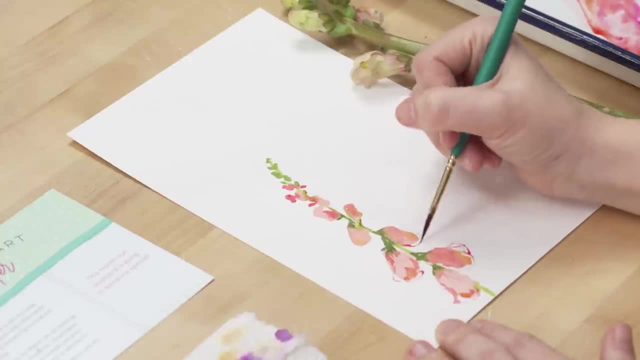 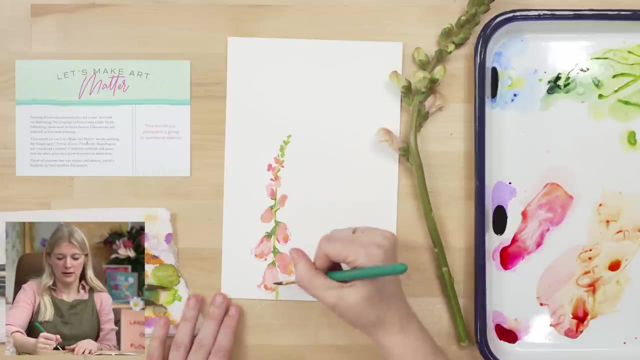 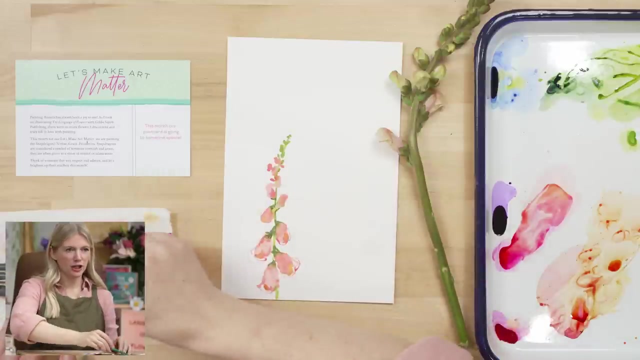 Now I'm going to go back over my pulleys and I'll mainly do that on the bottom ones, because the top ones are still pretty tight. Okay, just like that, That's a little bit of final snap dragging, So that is a good basic start. 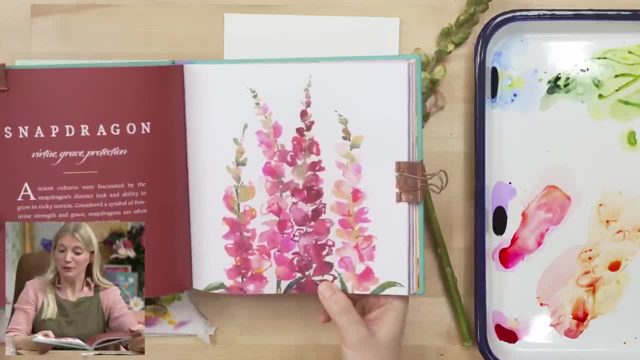 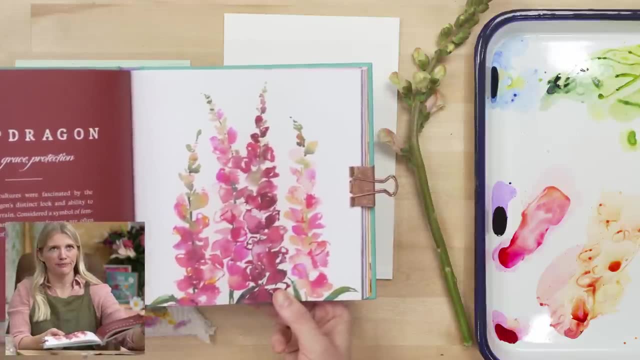 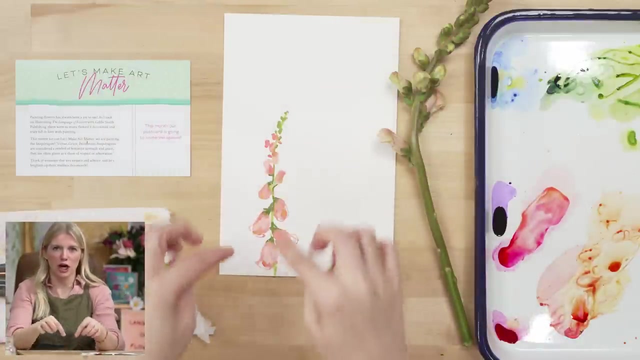 and then I want to show you the illustration I did for the book ¡language of flours¡ say a lot more flowers, which for me I think is a little bit more um, playful. So when I go to my postcard I'm going to take this and then, like, turn it up a notch and do a ton more blossoms on. 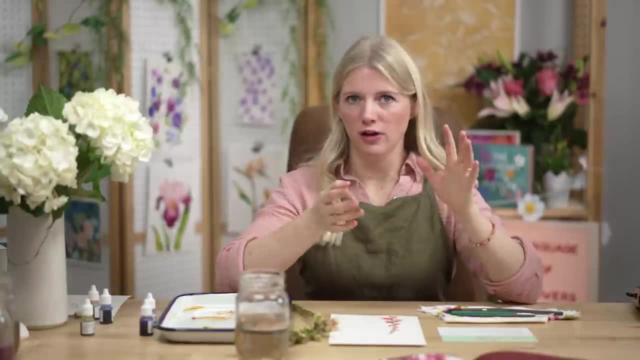 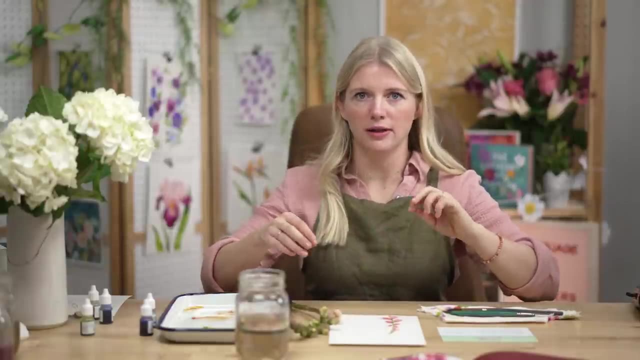 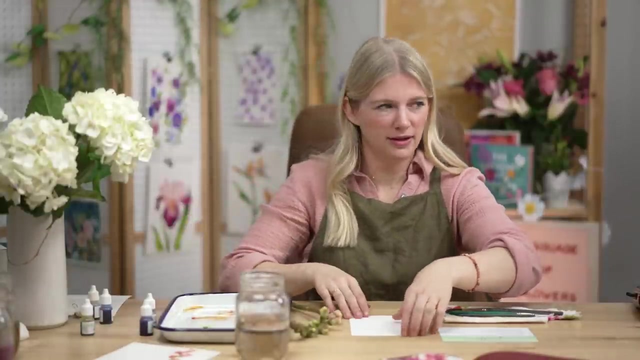 it Okay, But know that there is variation in all of them. You're it's okay If your snap dragon is a different colored, has different amounts of blooms on them. um is longer all of that kind of stuff. But if you just painted all buds just a bunch of green dots all the way up instead of 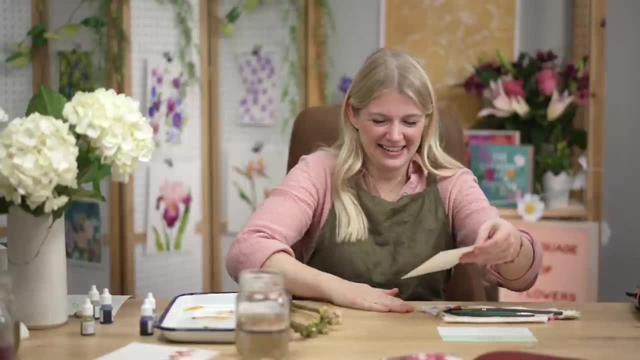 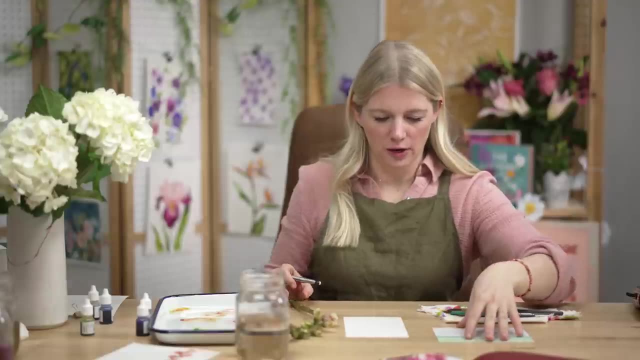 any bloom, you could do that. It'd look like a Brussels sprout, It would. So, um, whenever I approach a postcard and I'm thinking about: okay, I want to make sure my layout is good. I'm going. 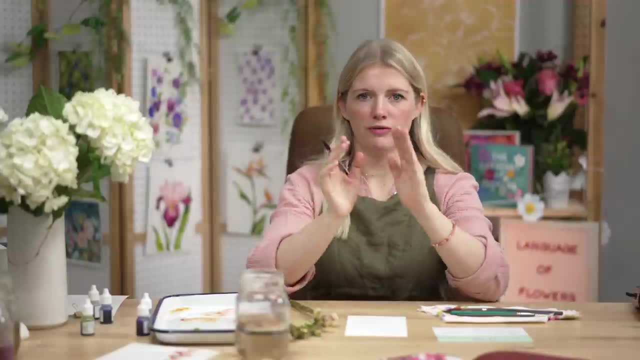 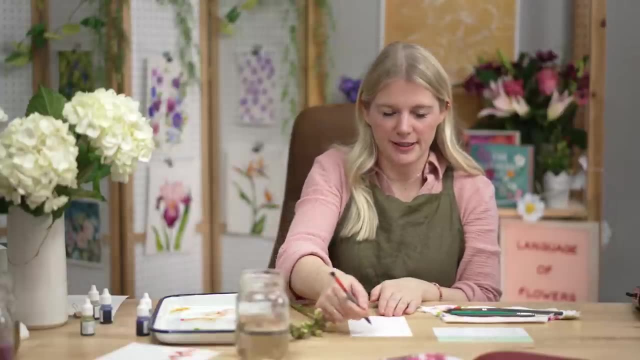 to turn it. I think about: do I want it horizontal or do I want it vertical? Because these are long, skinny flowers, I want to put my postcard vertical, which means standing up, So then I can really kind of accentuate with that. 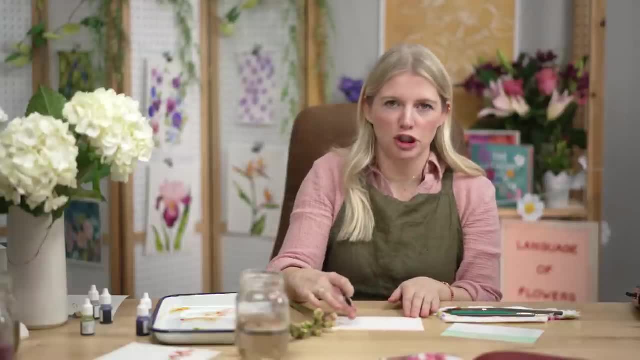 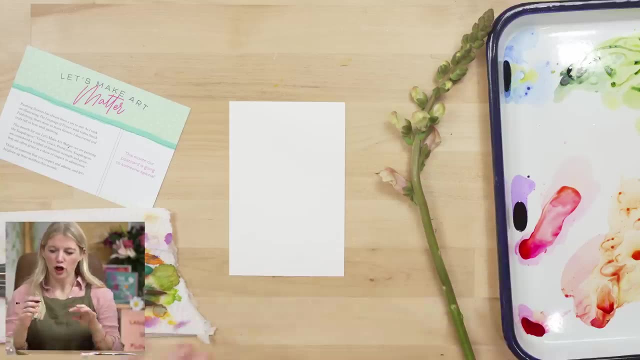 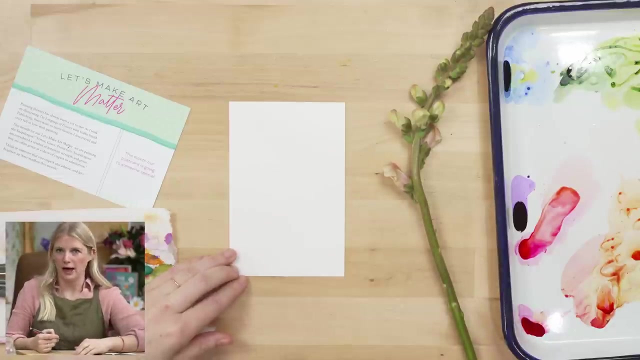 Length. If I were to turn it this way, my things would have to be pretty short and I'd have to do a lot more of them to kind of fill up that space. Now I'm going to think about the curve of them and, um, our brain is going to want them to be perfectly straight, but I don't, we don't want. 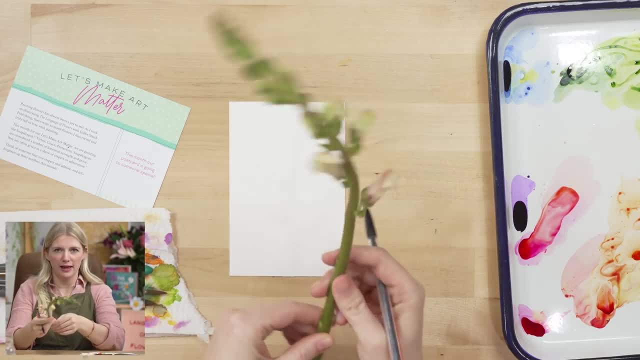 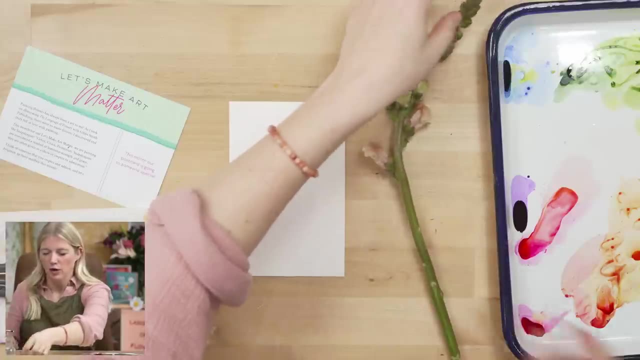 that, because that is not how they are. They have movement, They have a life and I want it to feel like it has slightly more energy, where, if you want it to be very static, and still that's when you do straight lines. but let's have, I'm going to have some of 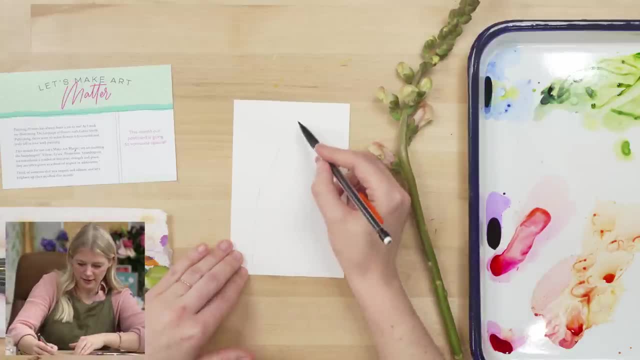 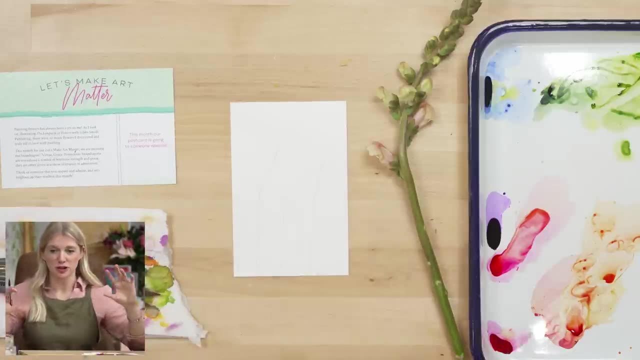 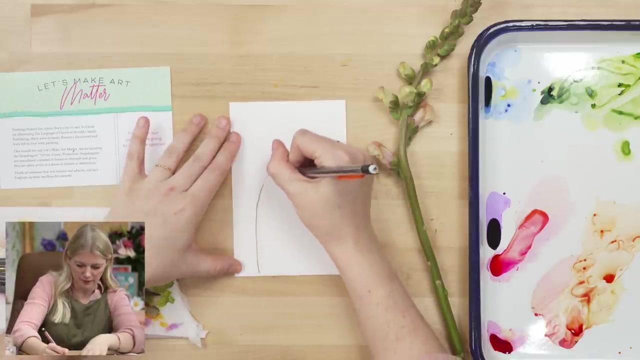 them curve this way, I'm going to switch up their lengths, Okay, And this is just basic. We're not going, we're not doing anything crazy, or I'm going to darken my line so you guys can see it better, But if you're sketching at home, don't do your lines this dark. 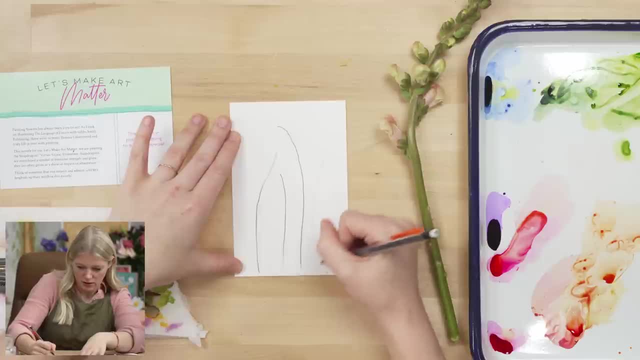 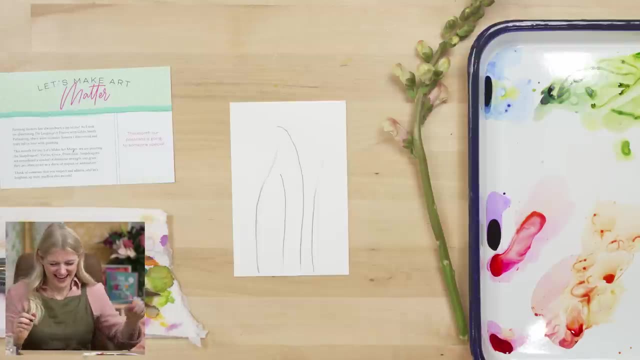 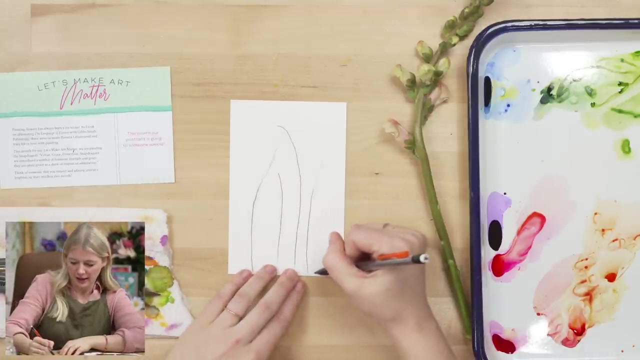 I guess you could eat the flower part, Really. Yeah, that's what the internet says, and the internet never is wrong. I always trust everything the internet says. Okay, So I'll I'll do four. You guys can do however many as you want. Also, they have these like little kind of long skinny leaves. 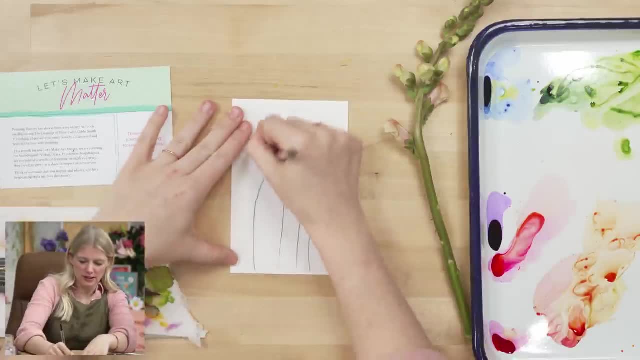 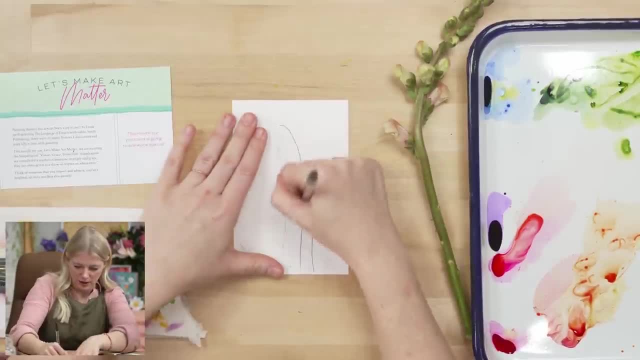 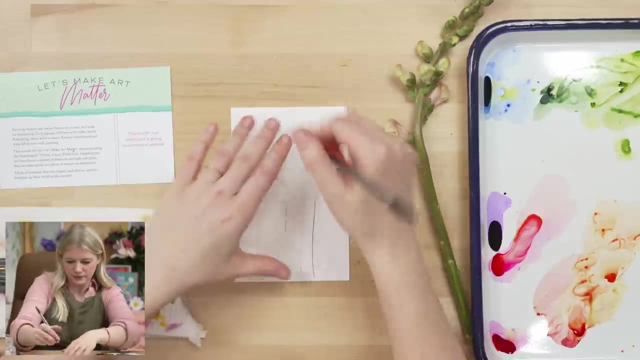 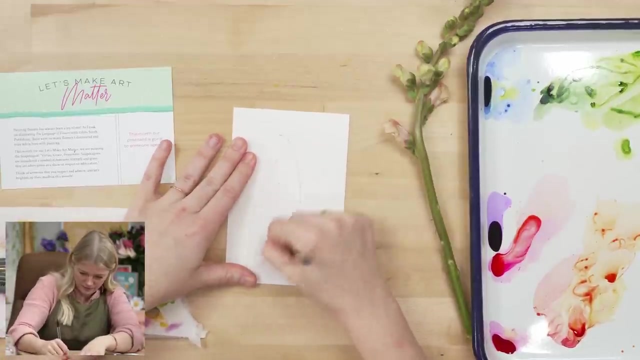 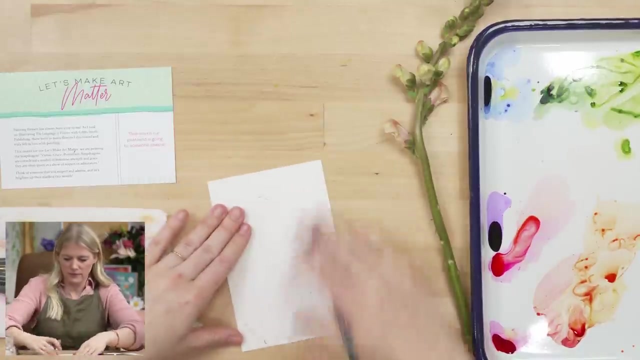 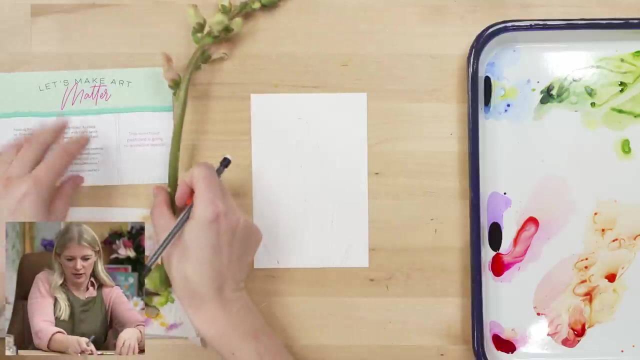 it's just not going to be able to cover those. So at least you guys could see what I was doing. And now I need to soften them so it doesn't take away from my painting. Okay, All right, Maybe I'll move this here. Is that better? 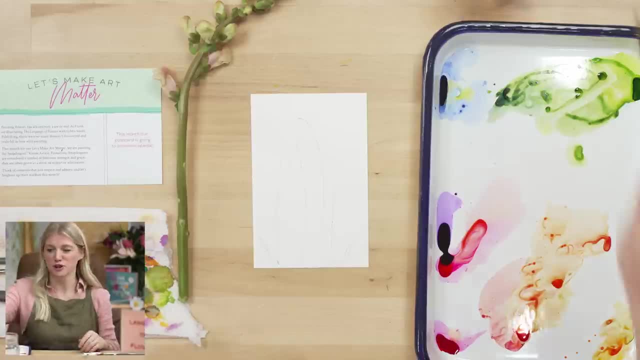 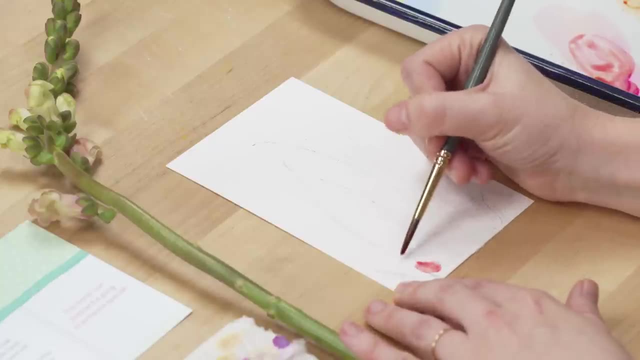 Okay, I'm going to use my six, but this is a smaller postcard, So if you have a smaller brush you would rather use, feel free. And then, um, this kind of like oval-y shape. Remember that the stock is three-dimensional. 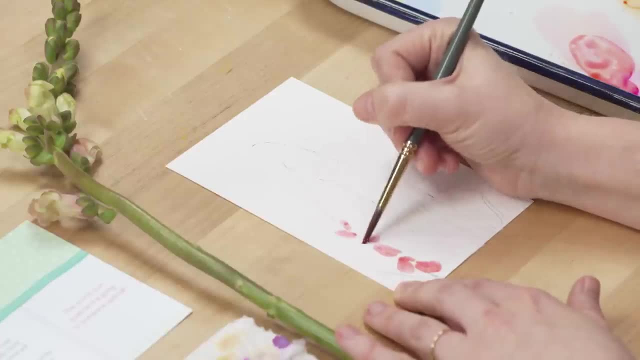 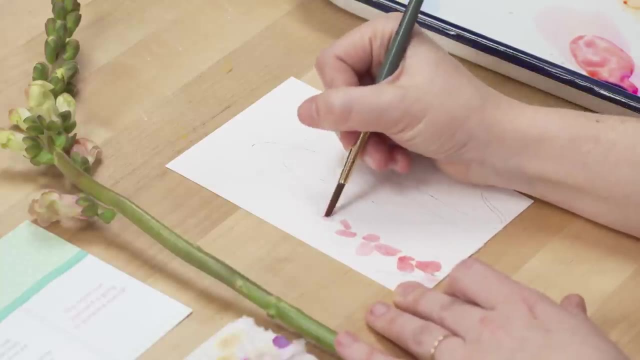 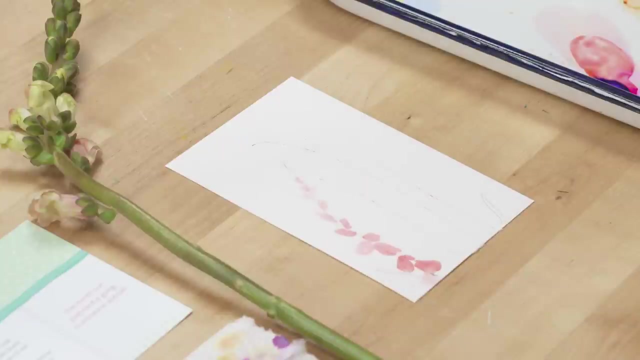 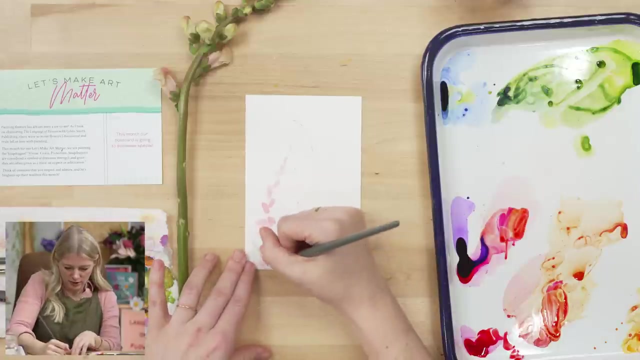 So there's some behind it. They can stick up, They can stick out. Allow yourself to add some water and then do lighter values. So whatever color you want to get that Me, I will do the lighter value ones as well, Okay. 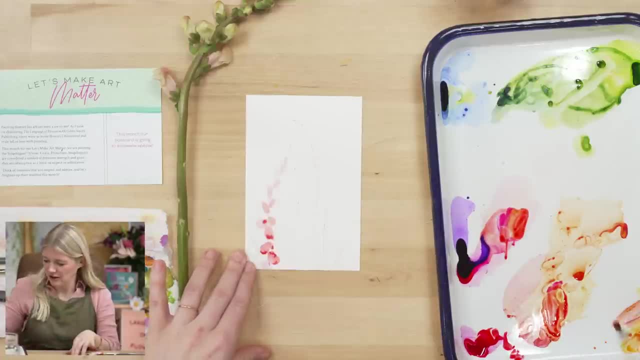 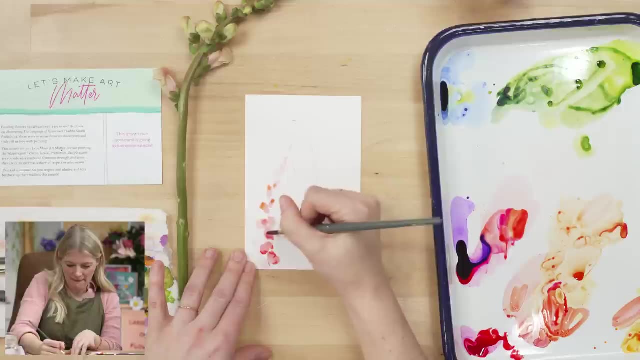 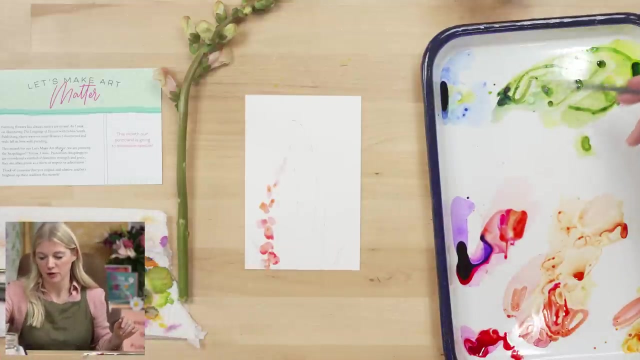 And then for fun, we can drop in some stronger color, Whatever, whatever color you like, It just gives it a little bit extra something. you know wet. I like to do this stem while it's wet because I like it when the green. 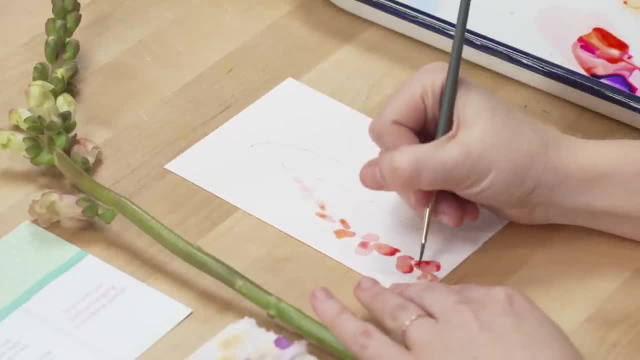 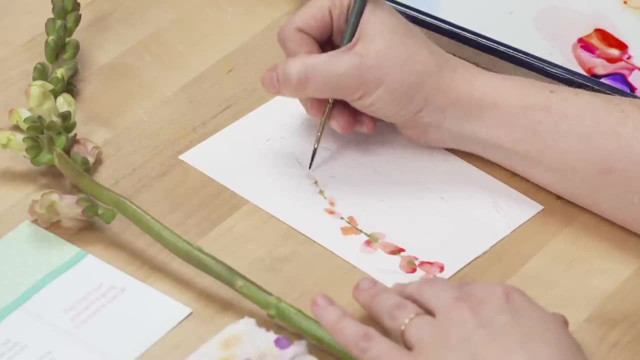 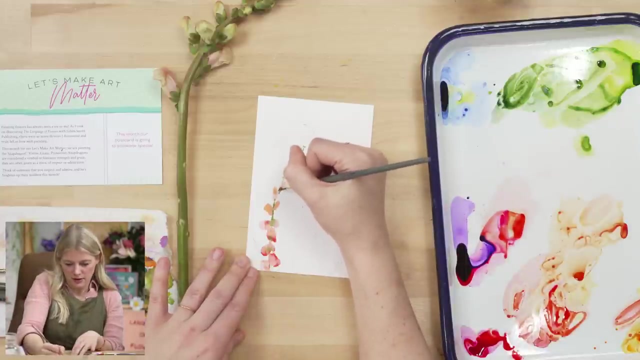 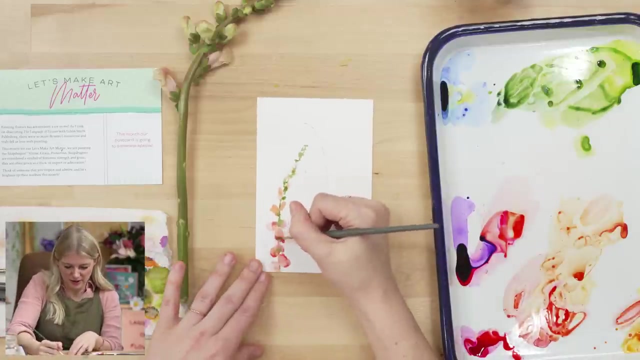 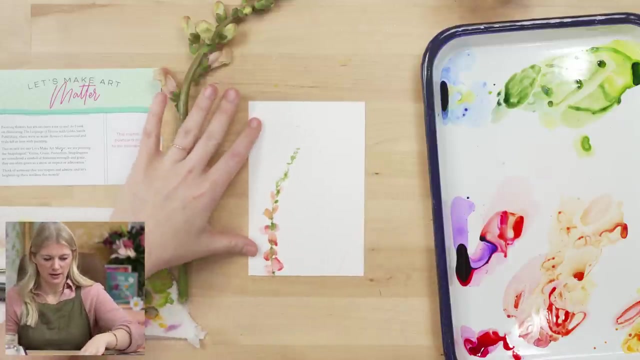 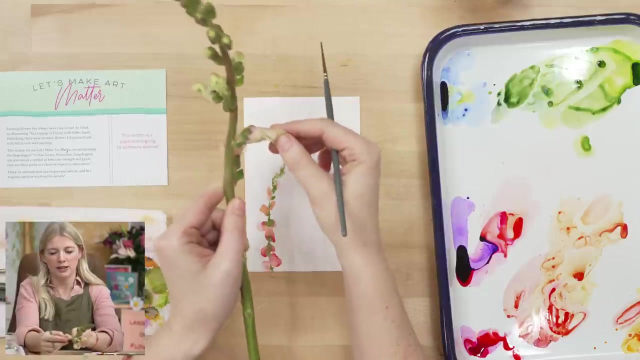 bleeds a little bit. so I'm just gonna basically just work around the blossoms, letting them kind of touch. then I do the dots at the top and the Brussels sprouts. we're doing the Brussels sprouts. it's stylistic preference. one but two- it's actually the green bleeding into the blossom can be. 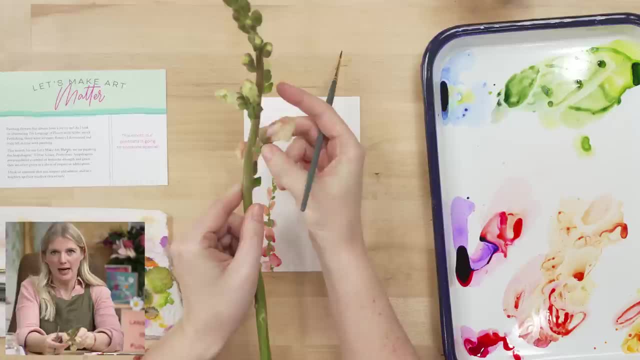 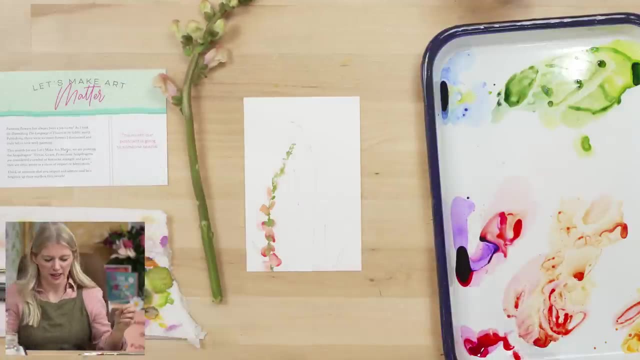 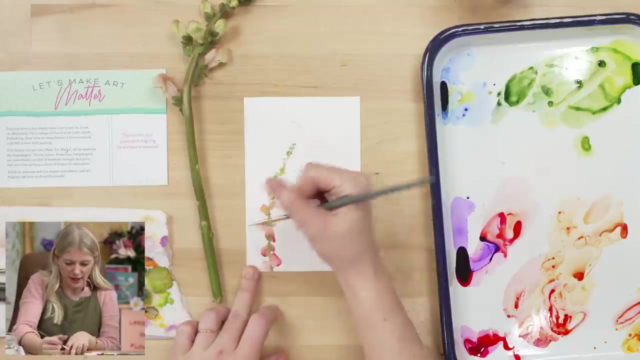 this bud that's opened up and actually, if you look a lot of times where the petals come out of a green area, there's a hint of green there too. so I just feel like I like it. and let's say: you do the green and it's just too strong. you can lift up some of that. 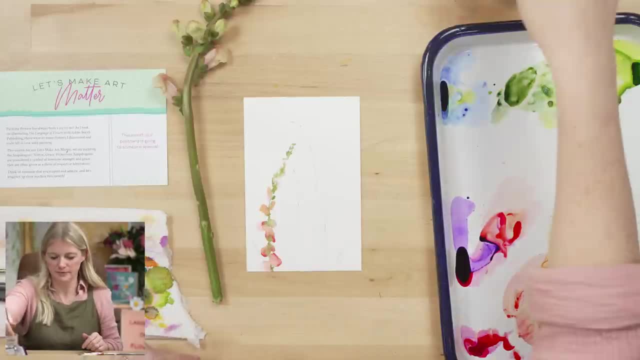 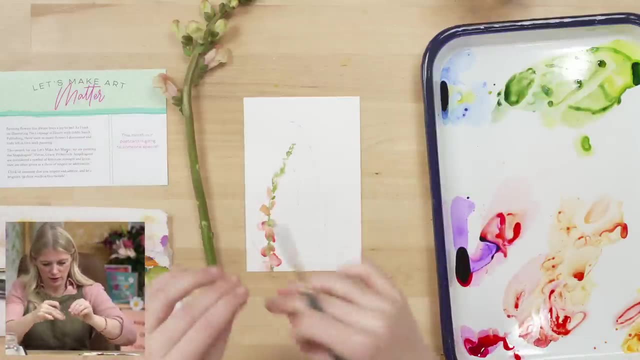 green and just kind of lighten it. it won't erase it, but it will soften. okay, that's one, and I'm not gonna do the detail lines of the little floofy at the end till I mean till the end. so I'm just gonna keep going. let's do like a full on. 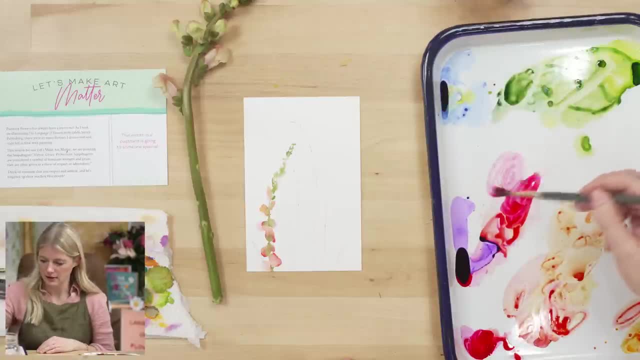 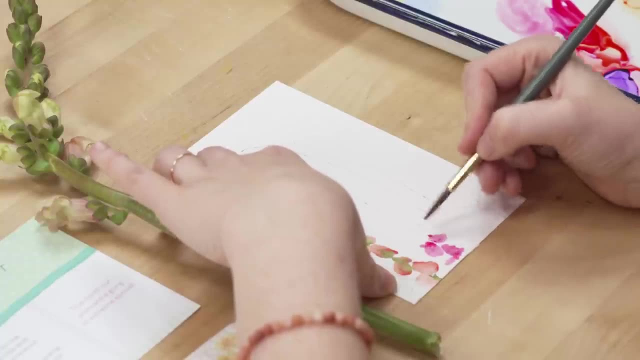 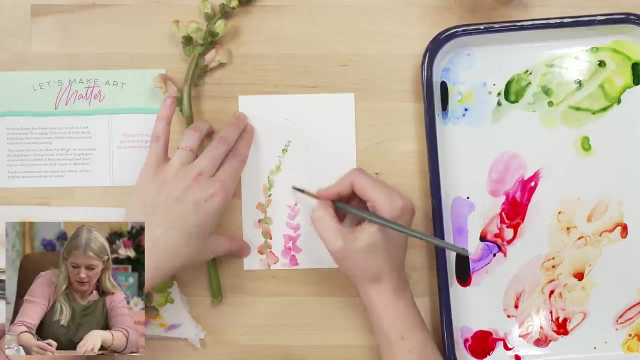 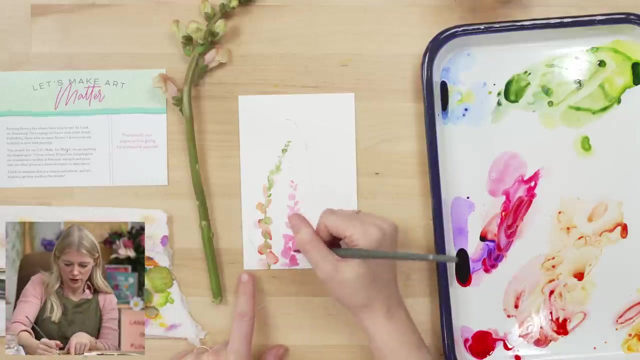 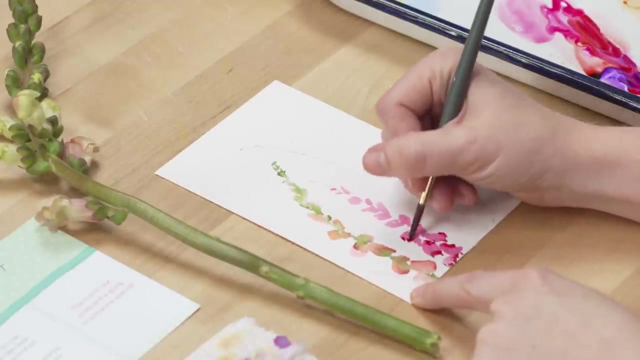 like bright pink. it's kind of like this oval shape, and it's okay if it's not perfectly rounded. let's drop in a little bit of color here and there. you can do it at the base or at the. you can do it at the base or at the. 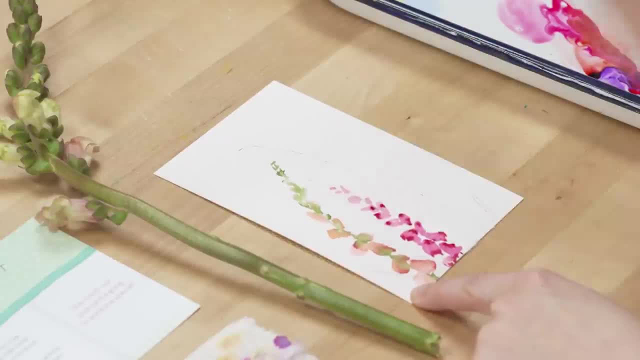 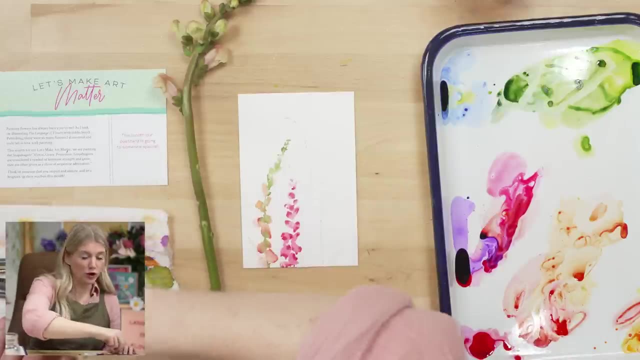 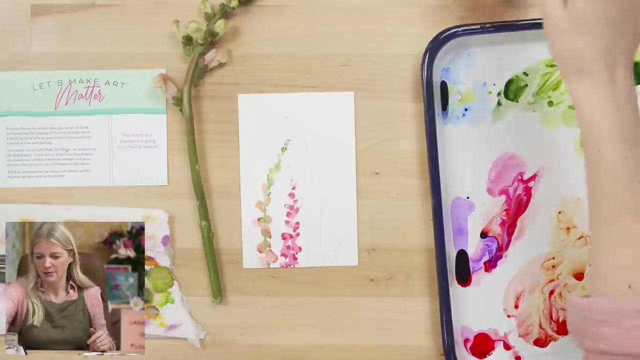 you can do it at the base or at the top. It's a good color, isn't it? Yeah, Now, if you don't like your green bleeding, then wait for it to dry and then add your green stem and just work around it. Same same thing, but it would just cut down on that green bleeding throughout. but I just feel like it creates this beautiful softness. 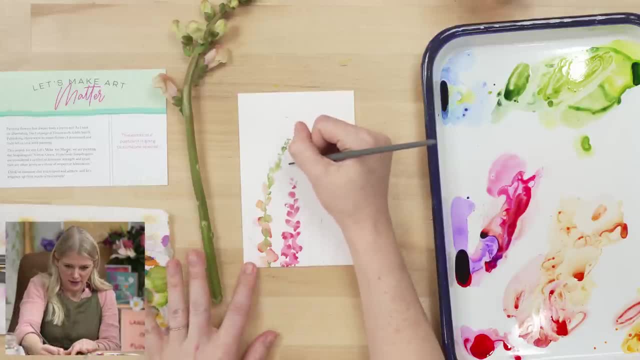 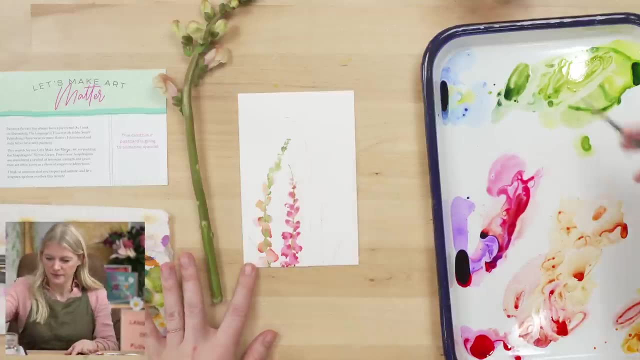 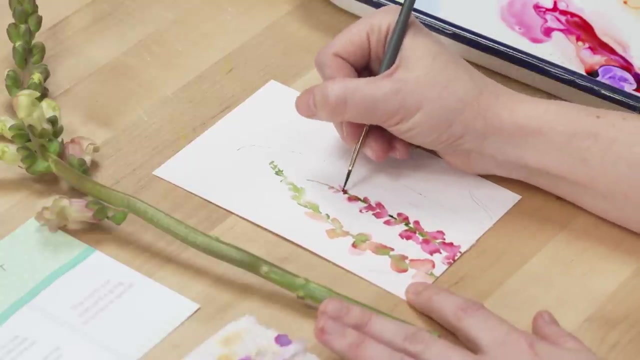 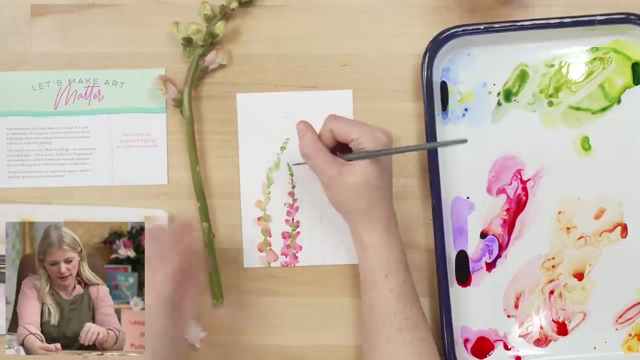 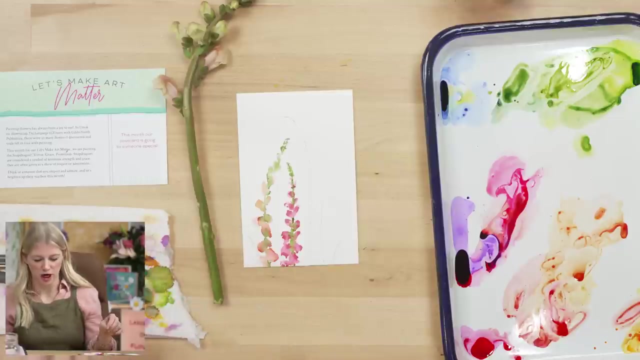 You can see that, So I'm a fan. Sometimes, in real life, I'm surprised by how vibrant and saturated flower colors can be. Mm-hmm, They look fake sometimes. Yes, Also, Snapdragon Stocks are obviously very thick. I Just love thin lines, though, So I narrow out the stocks on my own work. 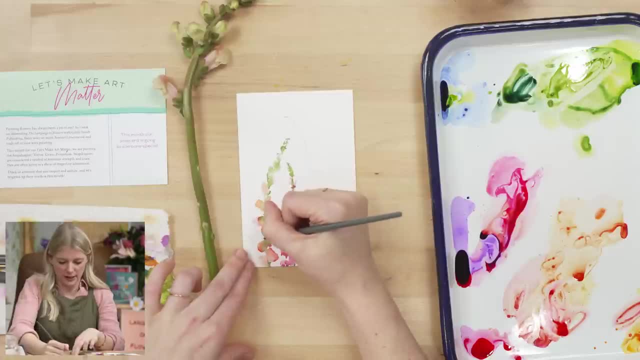 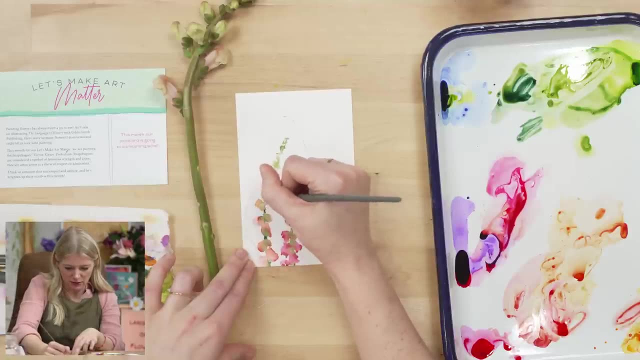 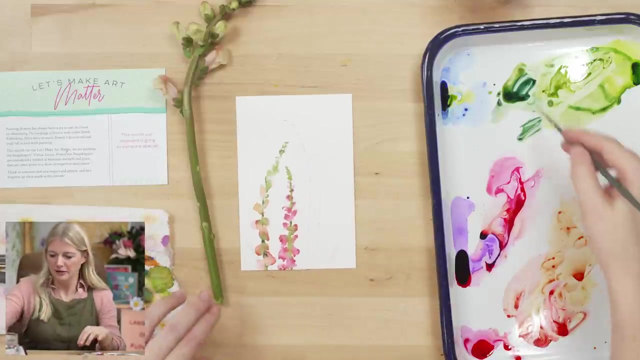 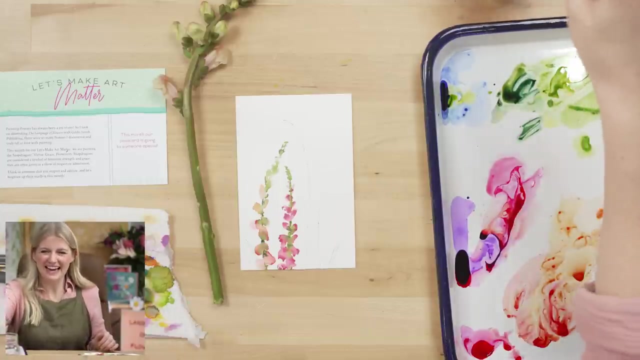 But if you're trying to recreate More realistically what it is that we're painting, you would want a thicker Stock. I just like thin ones. I think it just makes it feel Like a little bit more Elegant. I don't know, That looks like. Okay, let's do another one. 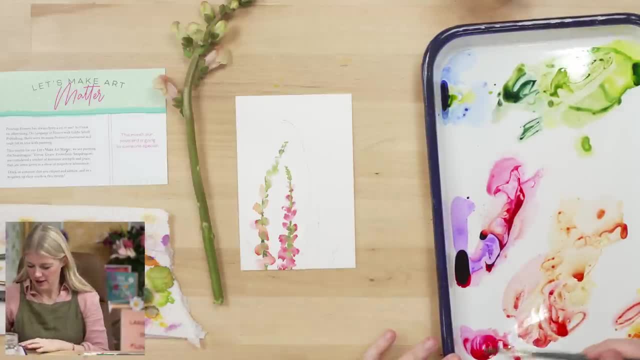 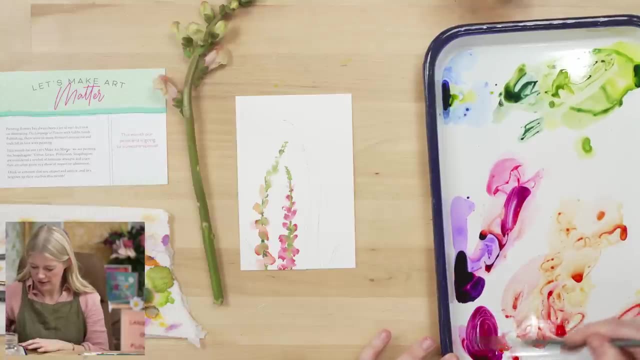 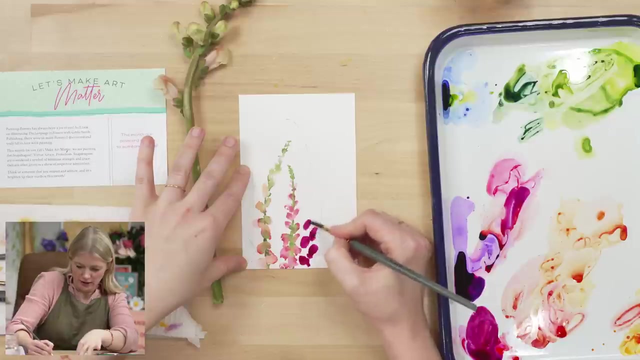 Let's do like a more, like a color. we did our iris, which is like a magenta violet mixture. oh yeah, this is a. these are just fast. just be loose with it. if you're paying yourself by the hour and you want to get the most out of your time, paint a bunch of snapdragons, man. i mean they can be if you're going for realism. 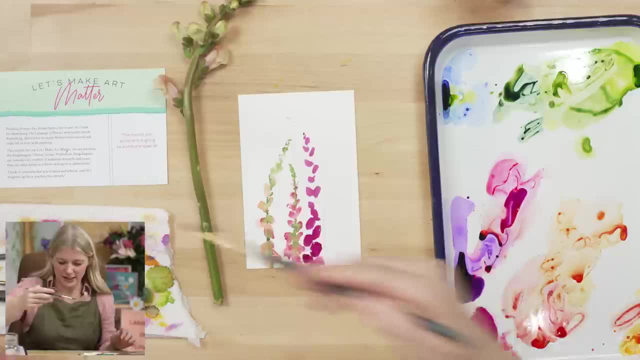 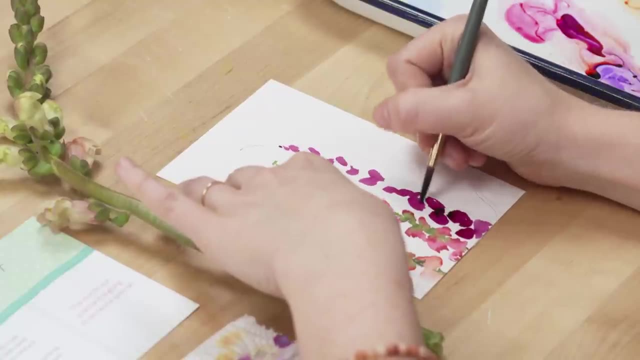 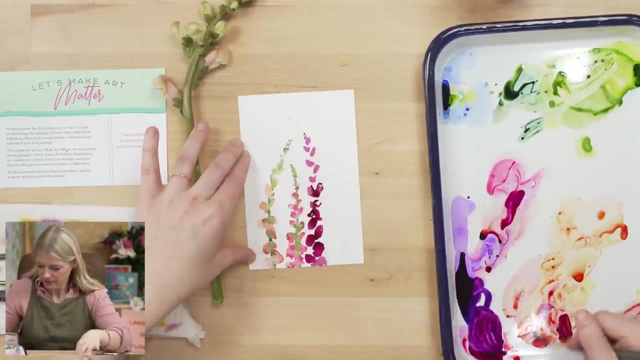 they can be complicated, but i like the looseness of them. i think. i think loose versions of them are just so lovely. i i that's my kind of favorite, one of my favorite flowers to paint, and this was one that i was painting um, while they were doing a photo shoot, and i was just like i just love. 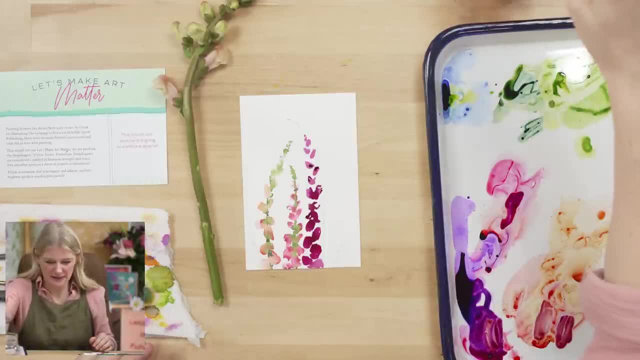 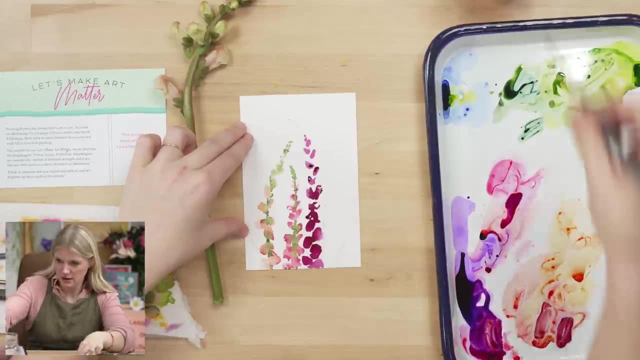 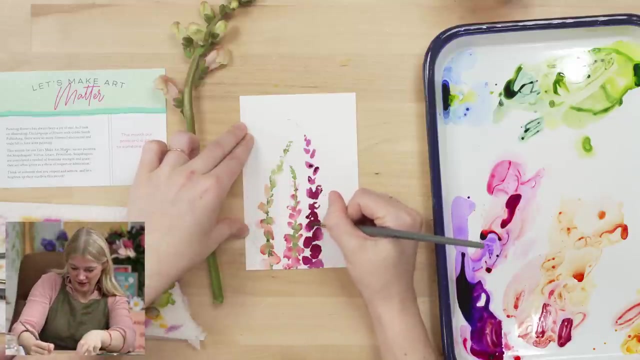 flowers. did you paint hollyhocks in your book? um, no, hollyhocks was not one of the flowers in the book. i feel like you'd like those. they have that loose quality that you could kind of paint quicker. well, i have done a hollyhock project for let's make art. actually i knew that. so if you 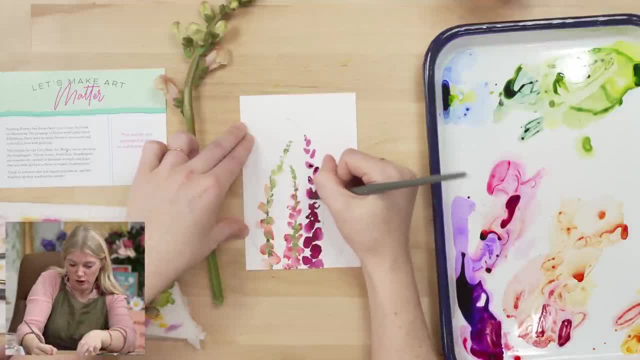 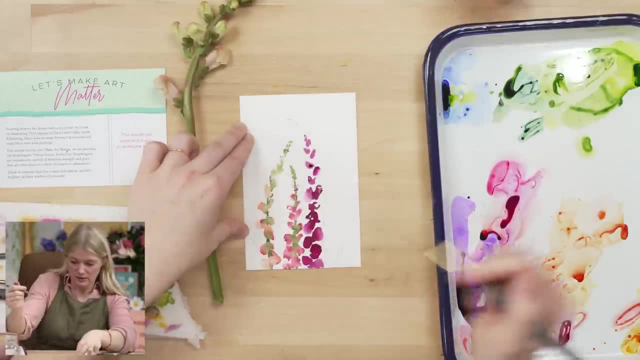 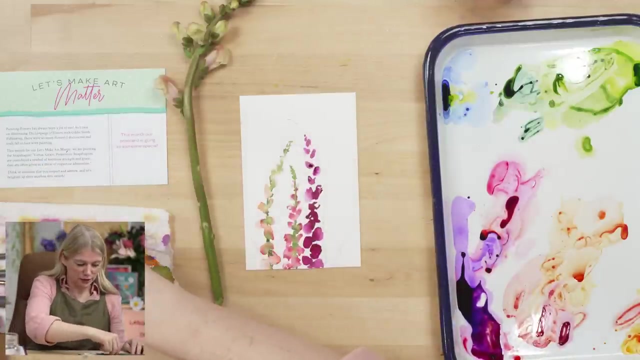 guys are interested in painting hollyhocks, which they do grow on a stock, similar to how these do, and they're beautiful. um, they're really fun to paint too. give a rough guess how many videos you up to. let's make art over three. i mean, i've done at least. 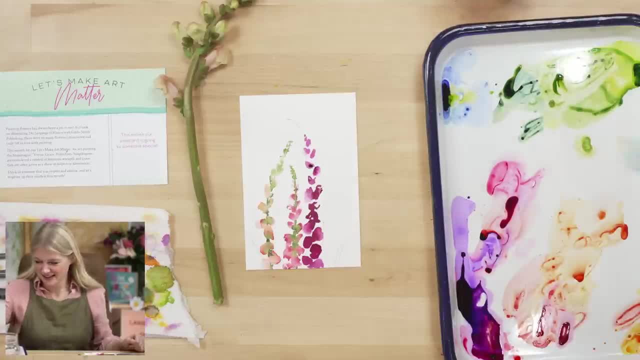 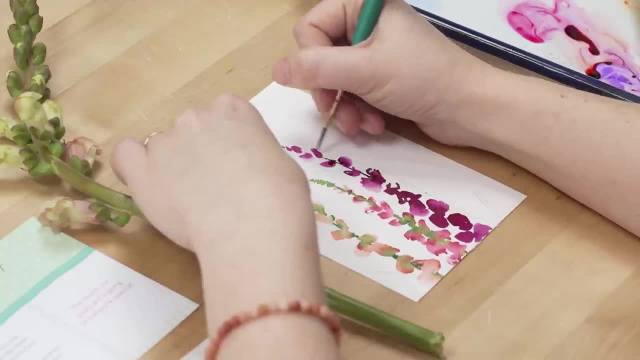 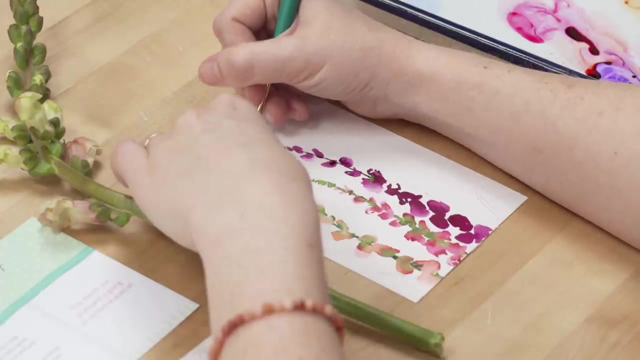 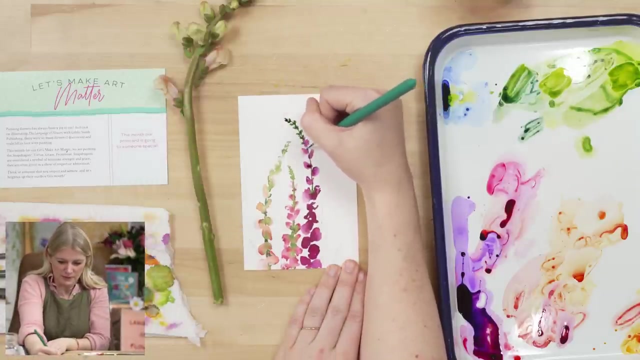 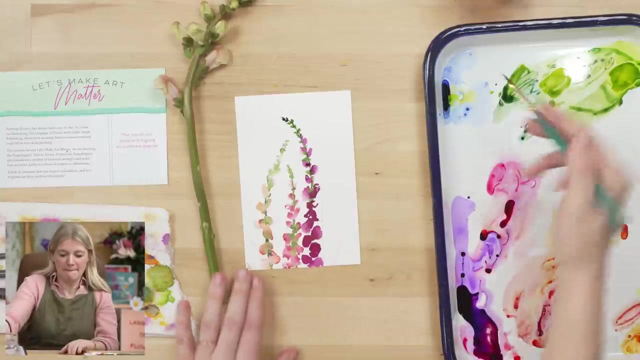 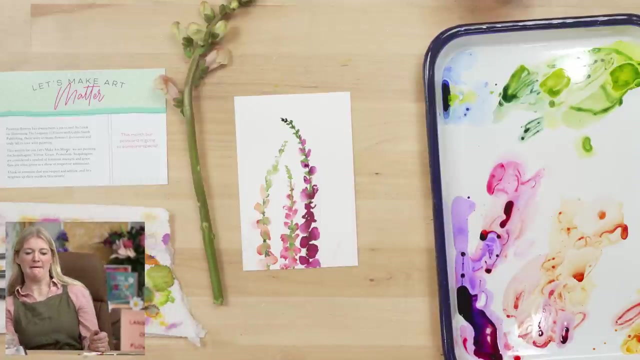 one a week since 2018 dang. so we're out 300 minimum, right? yeah, and that doesn't like there's some bonus in there and okay, now i'm adding the stock, let's add the buds. this one might have gotten a little too long, but that's okay. okay, i know i say it about everyone, but 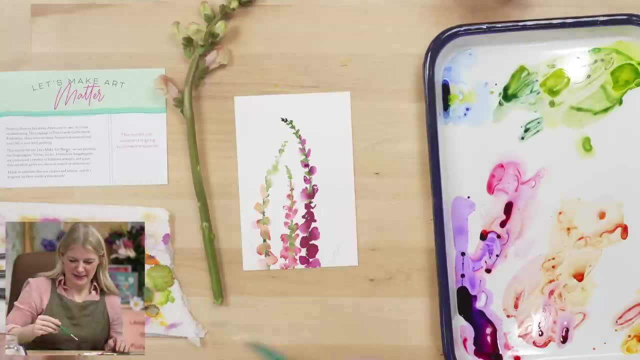 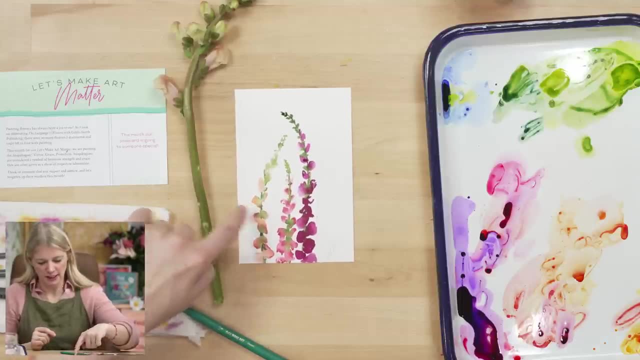 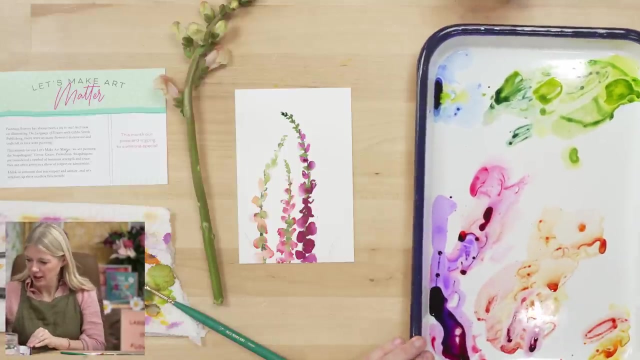 that one's not my favorite. and then now what i'm going to do on this last one. i'm going to make it more like this color, like more of a peachy pink. but i mean, this is your painting. there's even some like white and yellow ones, but i do need some fresh magenta to get that peachy pink back. 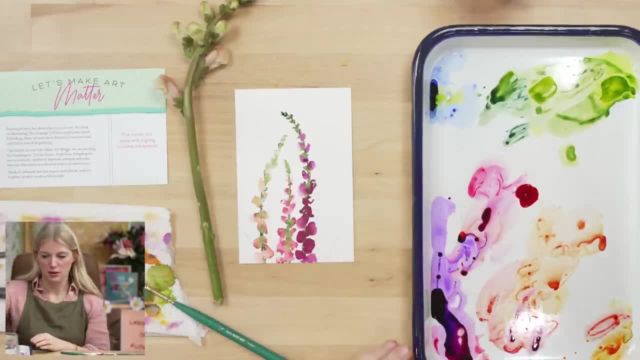 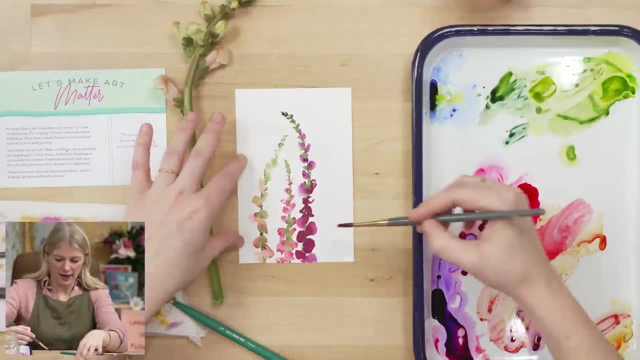 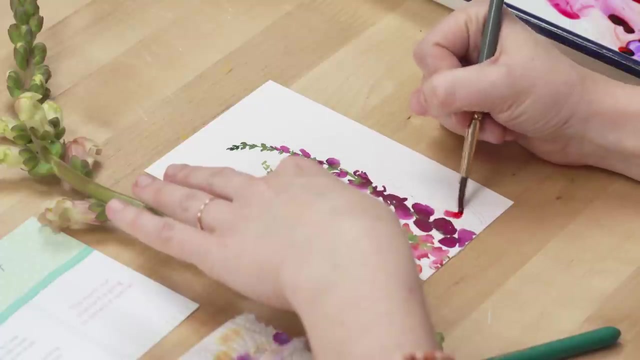 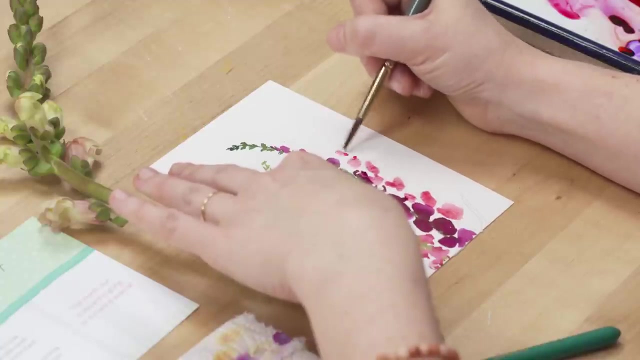 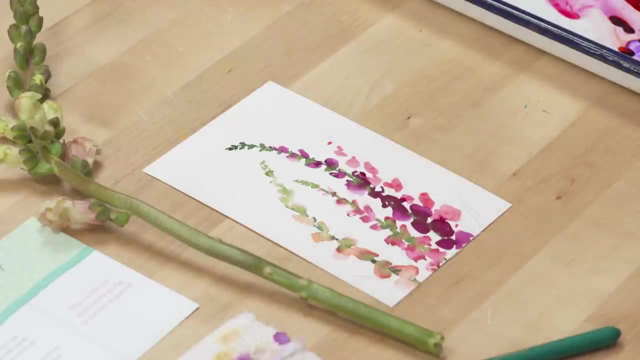 and maybe i'll have this one. the bloom start not as low, so then i can get some green along the bottom. so let's have them kind of start here and it's okay if they overlap with other ones. i kind of run into this one: let's drop in a little bit of. i'm gonna drop in a little yellow. 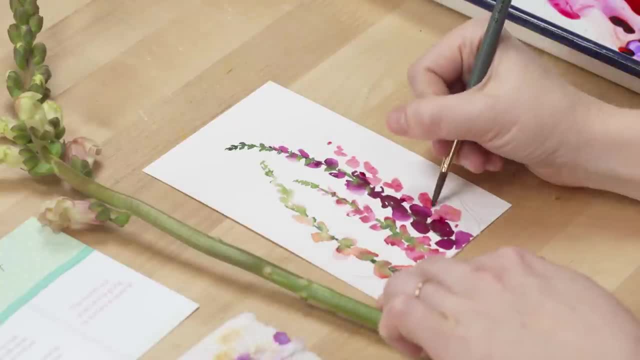 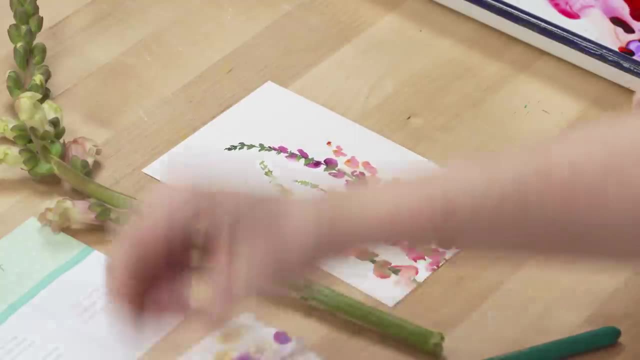 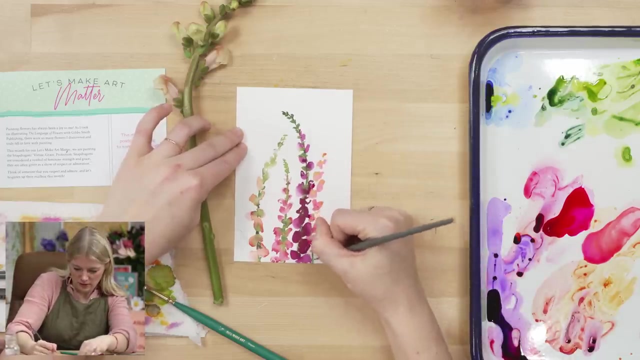 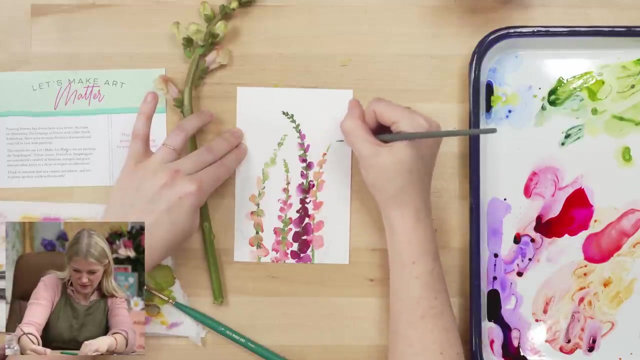 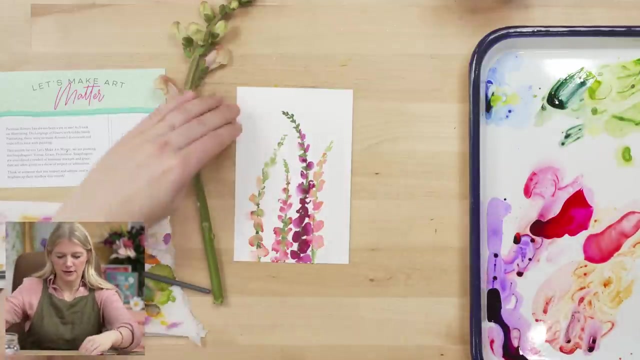 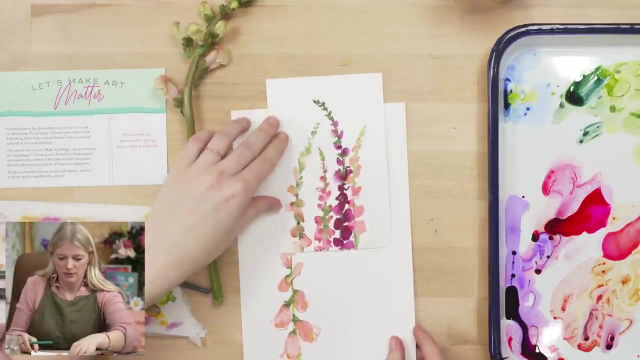 okay, you can use your two or your dagger for the stem. sorry, i'm not completing my thoughts here because i'm focused. okay, and actually let's use our dagger to do those long skinny leaves. i'm going to put a paper underneath this so i don't get my table. 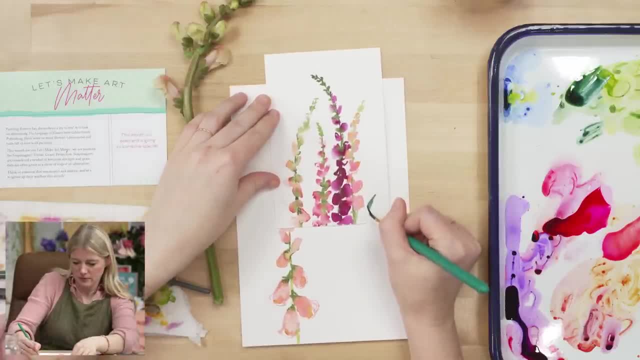 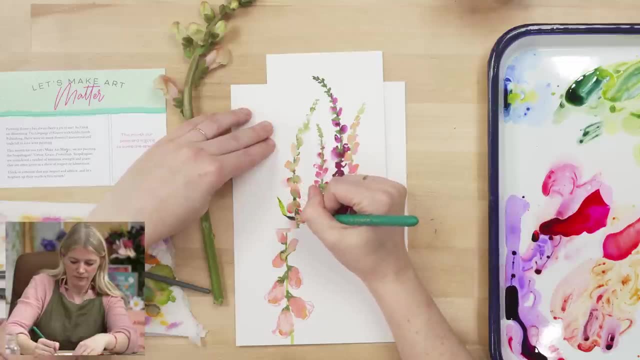 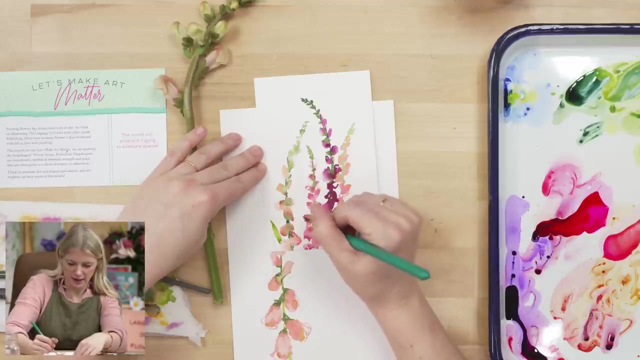 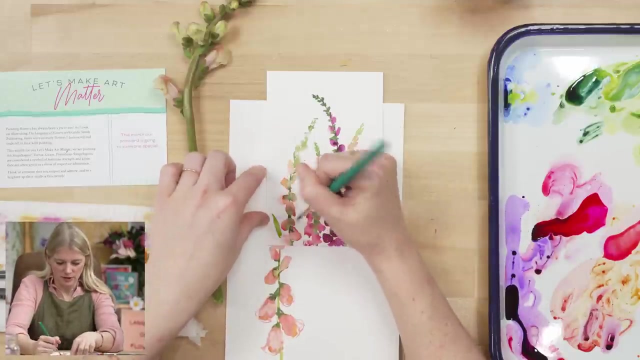 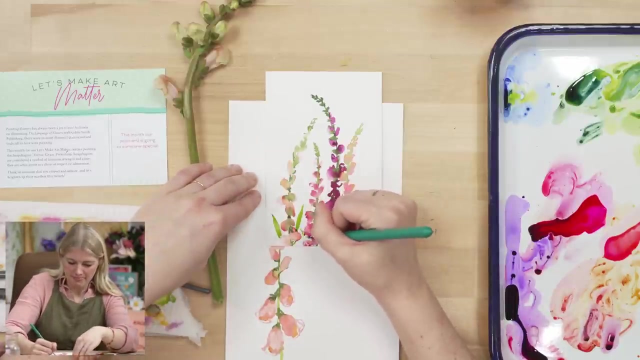 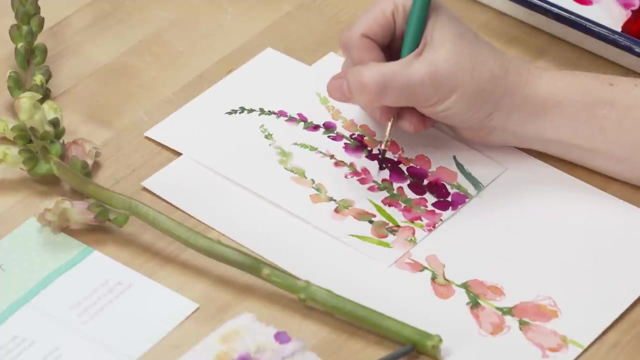 messed up and then, wherever you feel like it could use a little extra space- like maybe right here we can do another one, trying to decide if i want it coming out of this one or this one- i'm gonna have it come out of this one and then, if you want to do like an extra on some of these stems, you could do like a darker value. 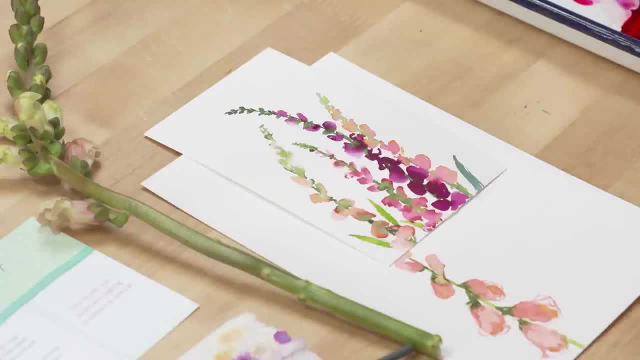 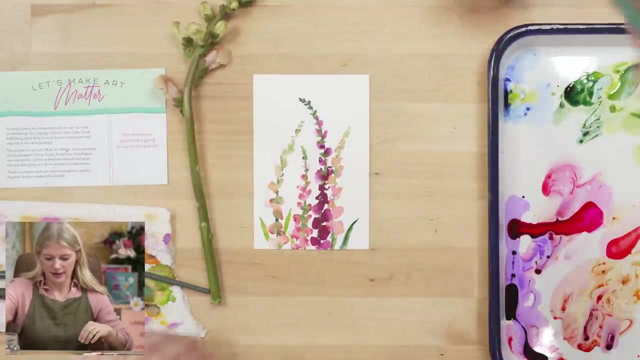 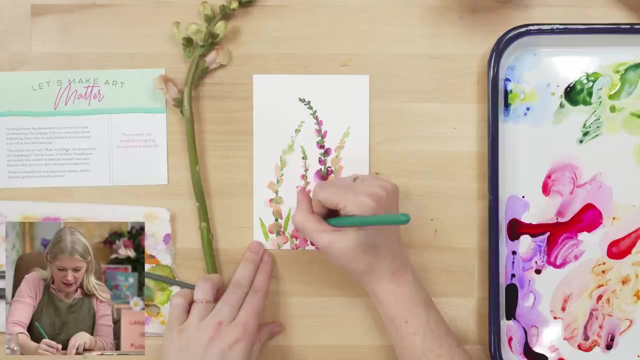 edge on some of them, just to give that a slight hint of dimension. okay, and now let's do our little detail lines. now, these are so tiny that we're not looking for a lot. i basically just kind of want to shape some of them to hint that there's like a little fluttery edge. just remember to use the same hue. 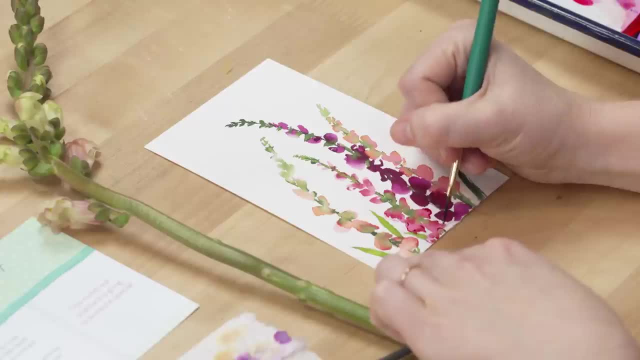 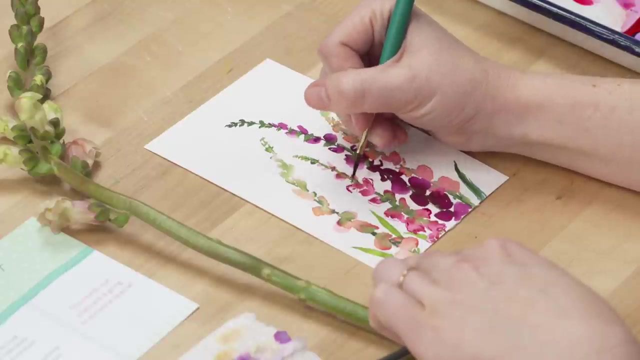 so i wouldn't be using peachy pink on the dark purple for these detail lines. you know what i mean, and i like to draw sometimes with my brush, especially with the dagger. it has such a fine point that i can kind of go outside what i've painted, because then they can really see it. 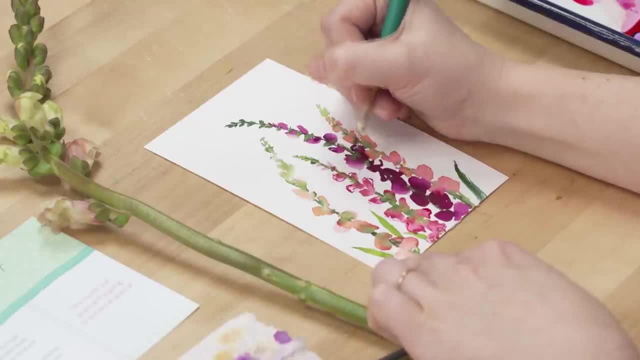 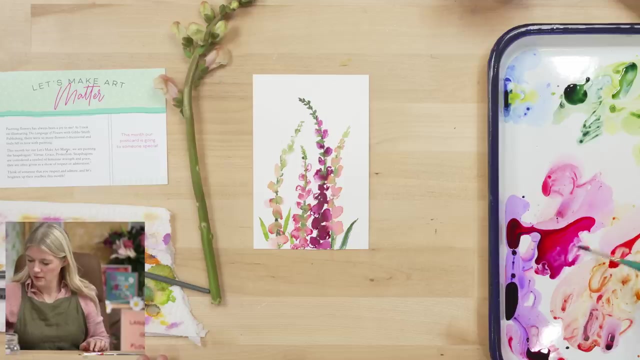 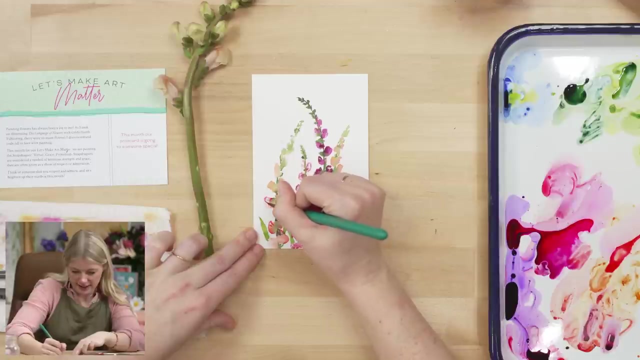 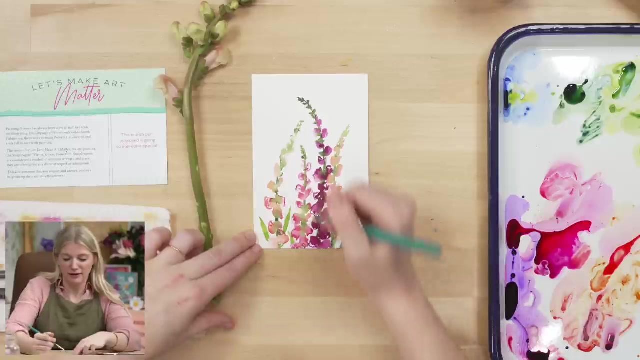 gives it kind of like a sketchy, kind of ink and wash look, which i'm a fan of personally, and basically i'm just kind of doing wavy lines, that kind of get a little bit white wider at the bottom, so so, so, so this actually was going to be one of the projects- um, like full page projects- and then i read what it stood for and i was just like you know what? that would be perfect for our. let's make art matter. let's do that instead. 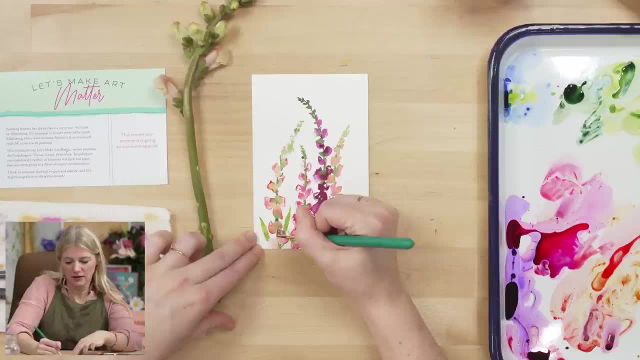 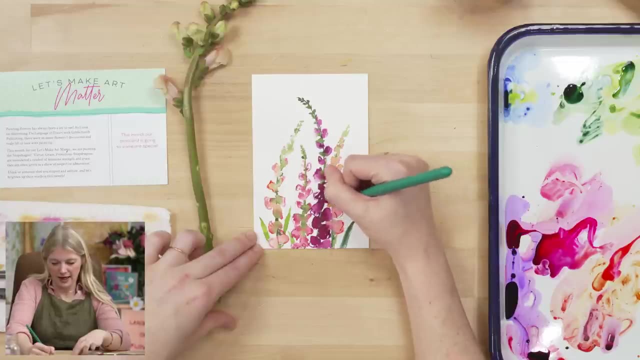 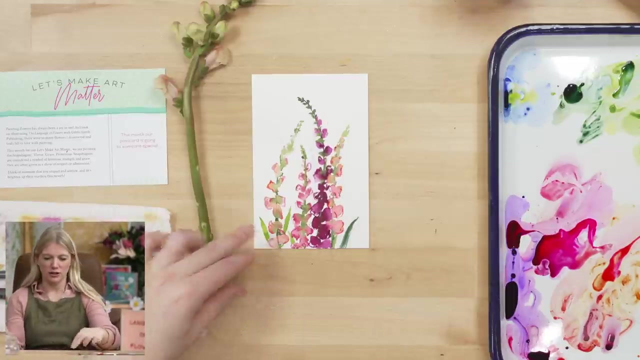 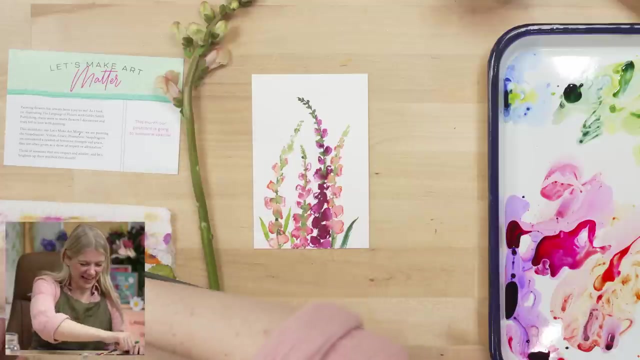 so so. so again, i'm just kind of like putting in some wavy lines on some of these. they're not super detailed, it's just like a hint of the shape and that's it beautiful. that's our snap dragging card, isn't it cute? i mean, the background is um. 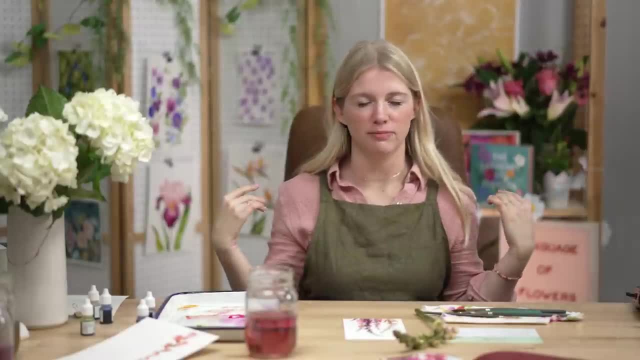 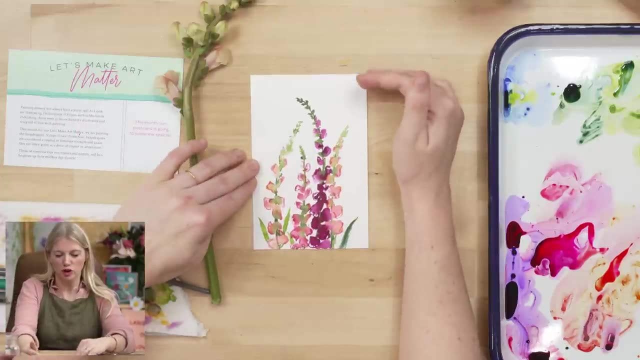 personally, i like a clean white background. i do it's just, but that's stylistic preference. so if you don't care for that, one thing that you could do is, before you start painting them, you could do a light blue wash with the and have it kind of transition to white, so you can start with like blue here. 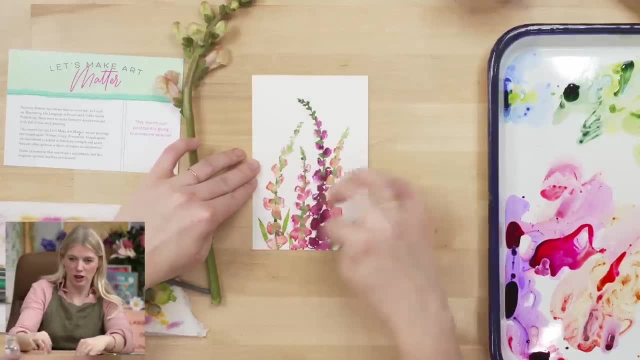 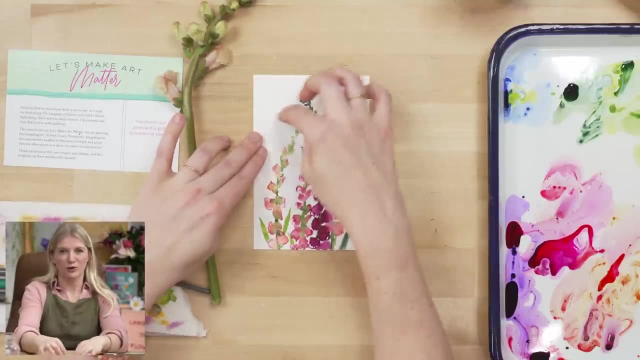 transition to a really, really light blue. so then that way, all of this gorgeous color would still show up, but you would have something along the top. you could also do a beautiful border, or maybe this is where you write a little note: okay, love it. um, i really hope you take the time. 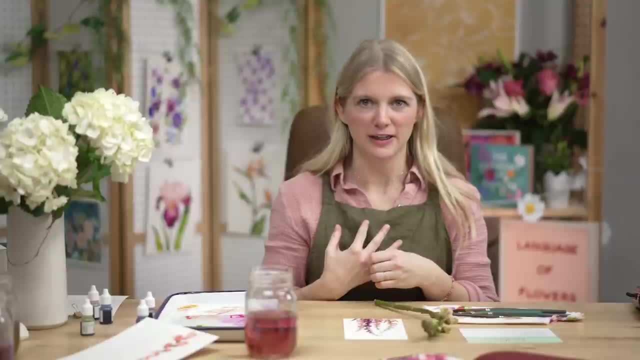 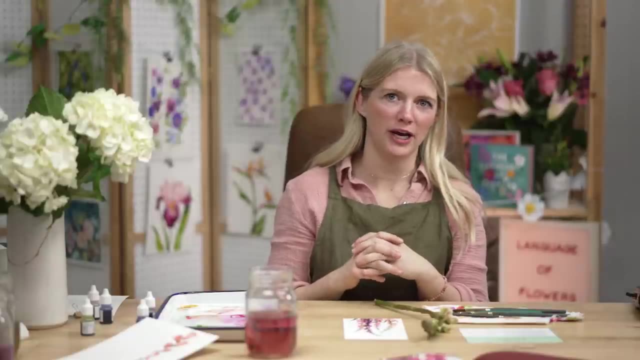 to do this- let's make art matter- is probably one of my favorite things that we do here, and i just think that there is so much value in letting people know that you care about them, and art has that power to do that. it doesn't have to be perfect, it's not about this frame: worthy painting. 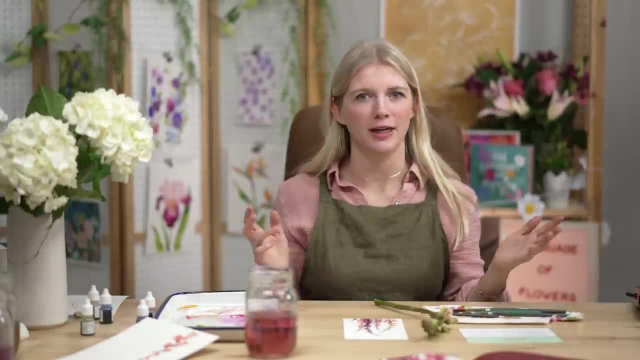 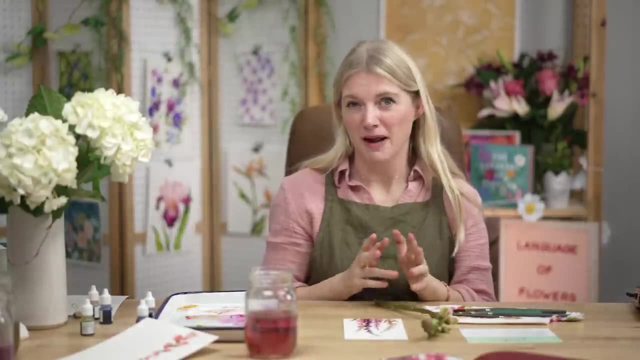 it's about making something for somebody and letting them know that you're thinking about them. that is it. that is that is the why that is what we're doing here. if there is someone you know that you think could benefit from a let's make art matter card, we have a nomination form on our 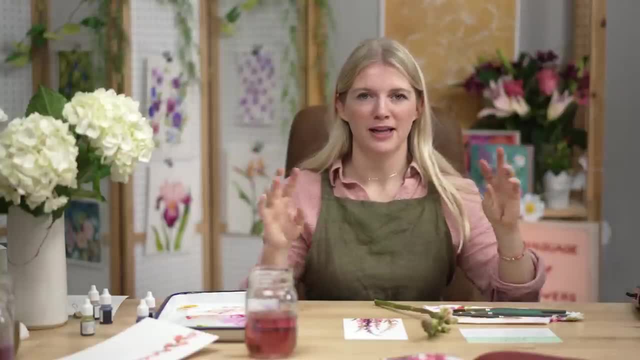 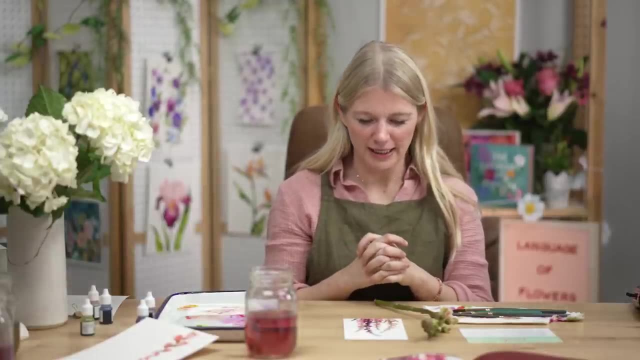 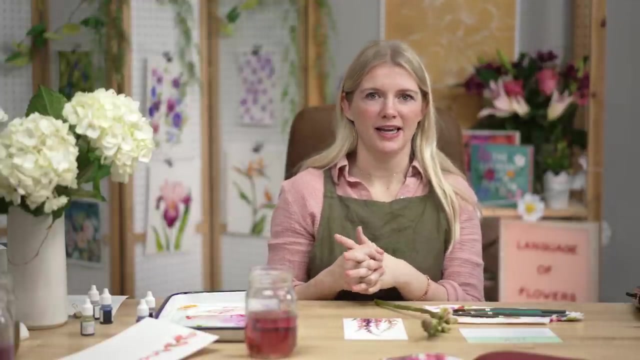 website. just go to letsmakeartcom, scroll to the bottom. there should be a nominate button there and, um, i just want to thank you guys for taking the time to do this. we get some wonderful thank you notes from people who have received postcards and i just want to say: it is not us, it is you guys. 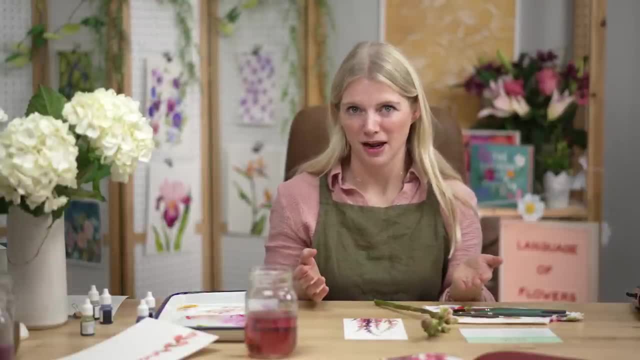 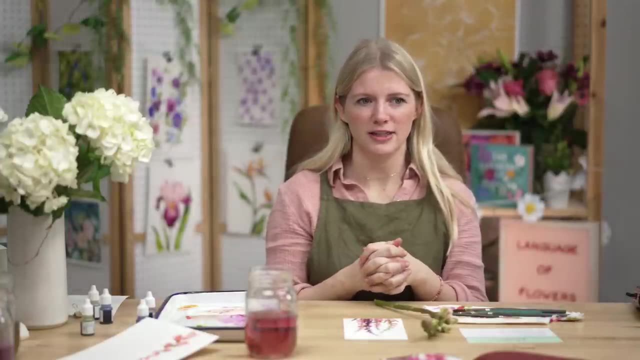 it is the people who take the time to actually paint something and put it in the mail- which is a very vulnerable thing to do- and if people appreciate the kindness and the generosity that does not come from us, that comes from you, and so i just want to say thank you for. 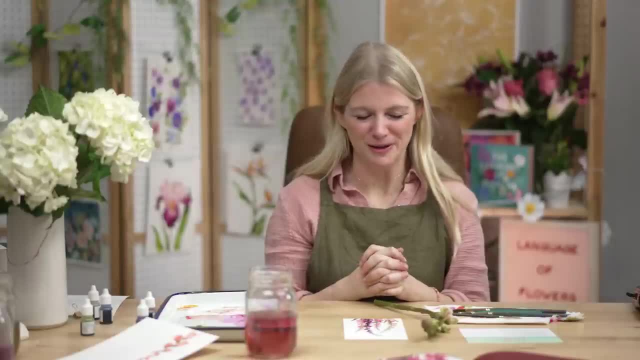 doing that and making people's day for doing that. so thank you for paying with me and i'll see you guys next time. bye.